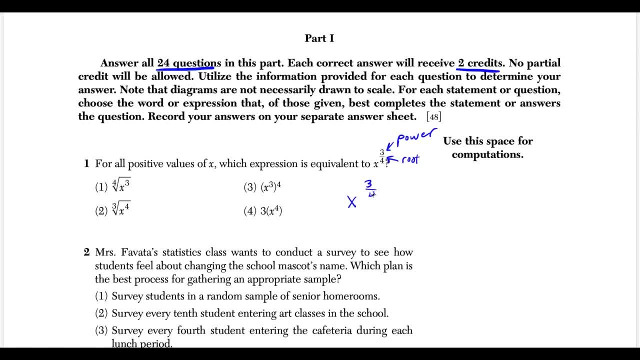 root. So if I want to transform x to the three-fourths power, I could rewrite this as the fourth root of x to the third power, like this. So now we just scan the answer choices and this is going to match choice one. Question two: we have Mrs Favada's statistics class and they want to. 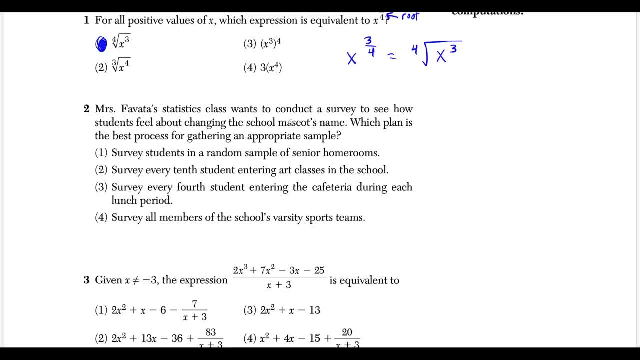 conduct a survey to see how students feel about changing the school's mascot's name. And now we have. which plan is the best process for gathering an appropriate sample? Now the key is: when you're gathering a sample, you want it to be as random as possible. So that's the theme with these questions. You want it to be. 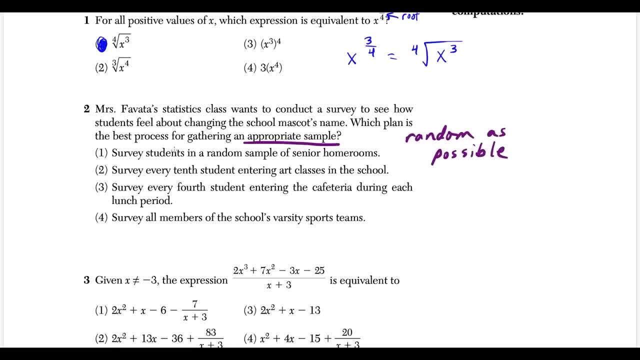 as random as possible. So if we were to survey students in a random sample of senior homerooms, that's not so random, because if you're at a high school, you have freshmen, sophomore juniors and seniors. So if you're only serving seniors, they're different than the other grades, So it's. 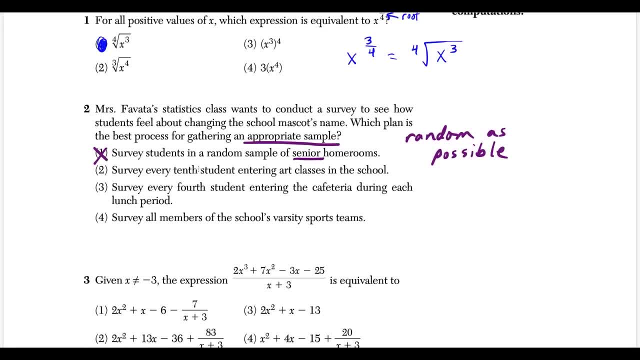 going to have a bit of a biased opinion. So now, if you survey every tenth student entering art classes, well then these are the students that are good at art, And if you're just mainly serving art students, you're not really getting a wide sample of the whole school. So I would say this: 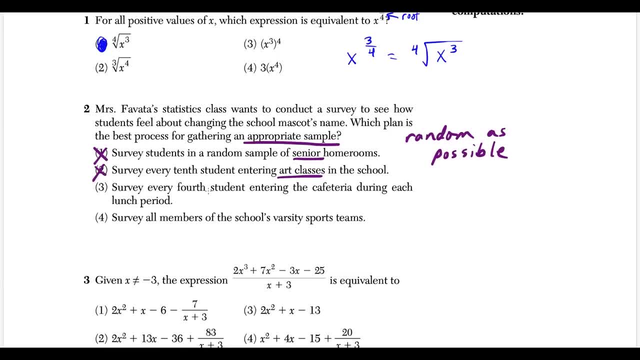 one is out as well, And now we're serving every fourth student entering the cafeteria during each lunch period. Now, this is as random as possible, because everyone in the school is going to eat food at some point of the day, So serving people in the lunchroom, you're going to get people who 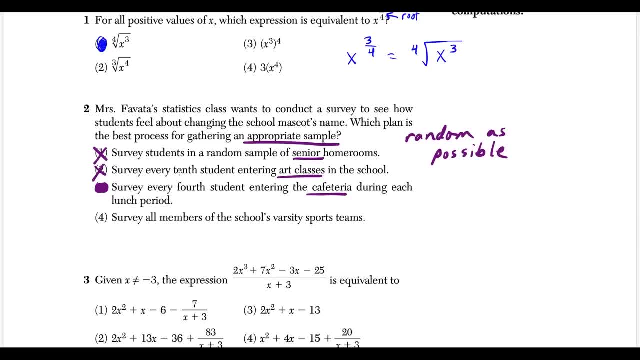 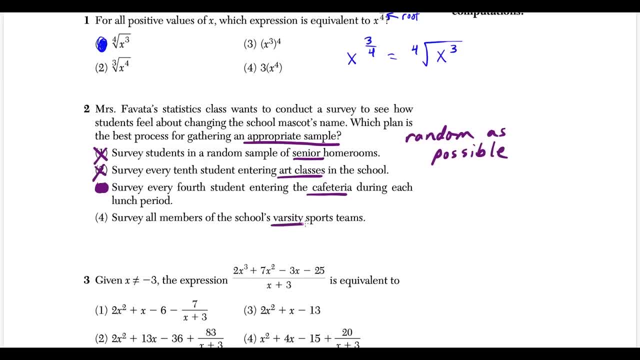 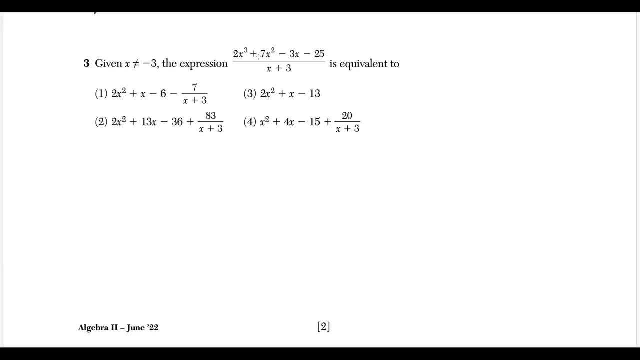 one. If we just survey members of the school's varsity sports teams, that's not that random. Three is the most random, So that's our answer. So question three: we have given x is not equal to negative three. We want to see what is this expression equivalent to. Now they have to specify. 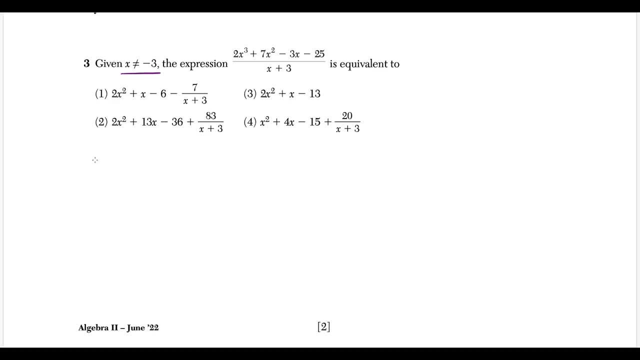 that x is not negative three, so that this is not undefined. And for this we're going to do, we're going to go ahead and do the long division here. So we have two x to the third plus, we have seven x squared minus three x minus 25.. So we could also do synthetic division here. But I think 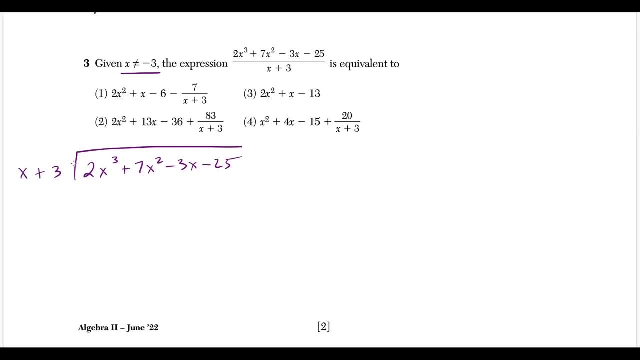 this is the more popular one, that's more widely taught across schools. So what we have is we're going to just do the leading terms here. So we're going to say x goes into two, x to the third, two x squared times. So right away I'm ruling out choice four because there should be a two. 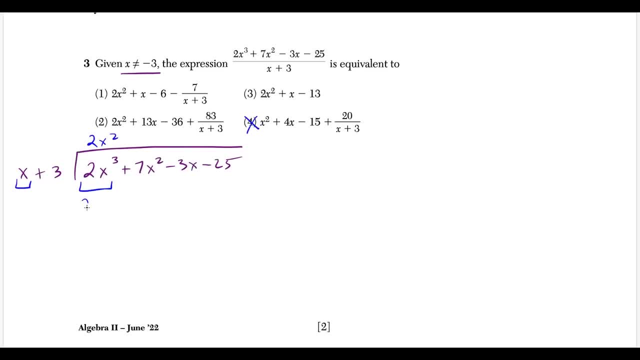 x squared in front. And now, when we distribute two x squared times x is two x to the third, And when we multiply it by three we're going to get six x squared. And then what we do is we subtract this row from the previous one, So these terms cancel. 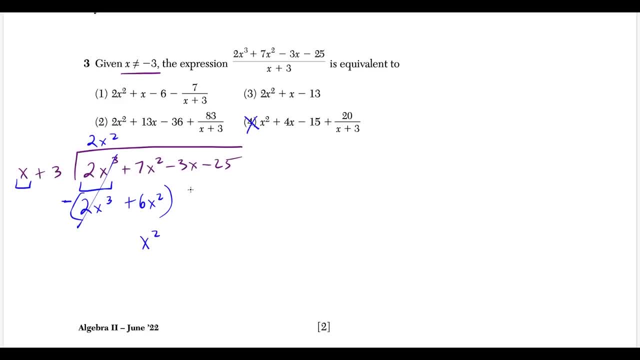 And then seven minus six is going to give us one. So we're going to have one x squared, And then we bring down the minus three x And we start this process all over. So now we're asking ourselves how many times is this x going to x squared? And it's going to go. 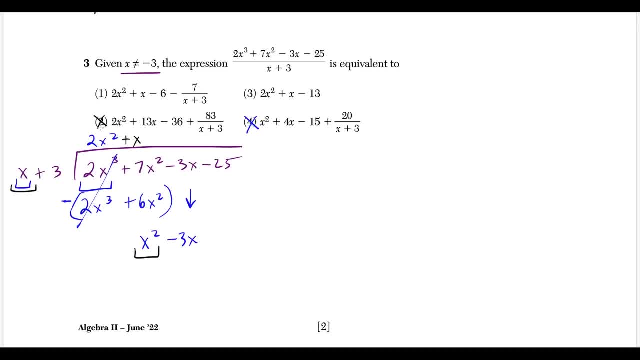 in x times. So right away I get rid of this one because it has a 13 x. So now it's between choices one and three. And now we distribute: x times x is going to give us x squared, And then x times three is going to give us three x. So now we subtract And notice here: 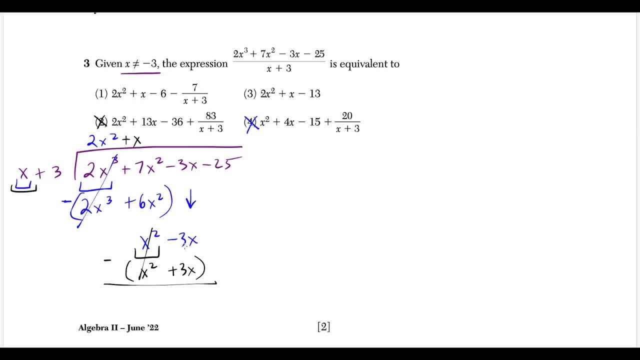 when we subtract this time, x squared minus x squared cancels, But we're gonna have minus three x. minus positive three x is going to give us minus six x, And then we drag down this minus 25 here. So now we're going to do this once more, Except this time what we have is x goes into minus six. 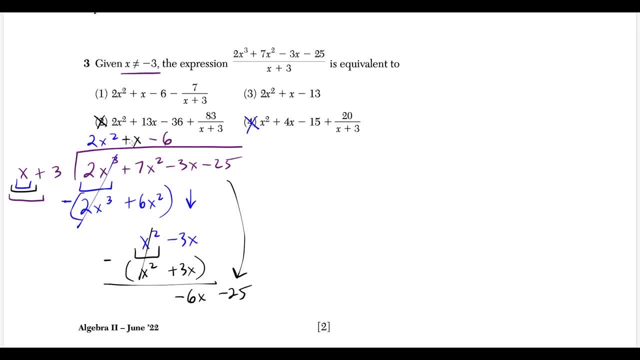 x, it's going to go in minus six times, And if we do minus six times x, that gives us minus six x, And if we do minus six times three, that gives us minus 18.. So now we're subtracting this row from the previous And we 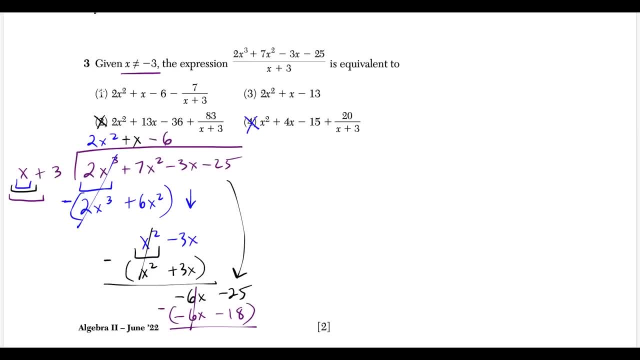 just have to pay real close attention here to the remainder. But look at this step: here I'm going to go with choice one, because, notice, choice three has a minus 13,. not a minus six. So this one is out. But just to verify here that this does check out: if you do minus 25,, minus minus 18, that 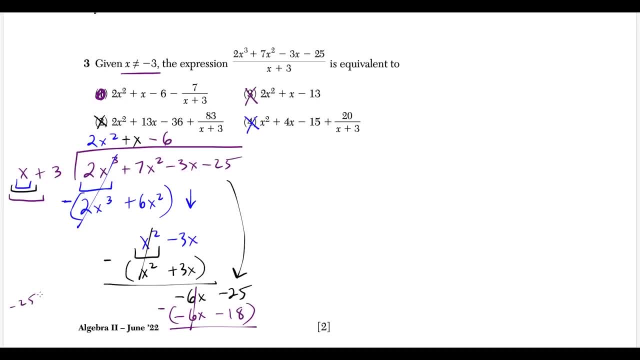 becomes a plus 18.. And if you just think about it, minus 25 plus 18 works out to minus seven. So this is our remainder. we have a remainder of minus seven. So I would have minus seven divided by. we were dividing by x plus three. So that's why this is definitely matching up with choice one. So 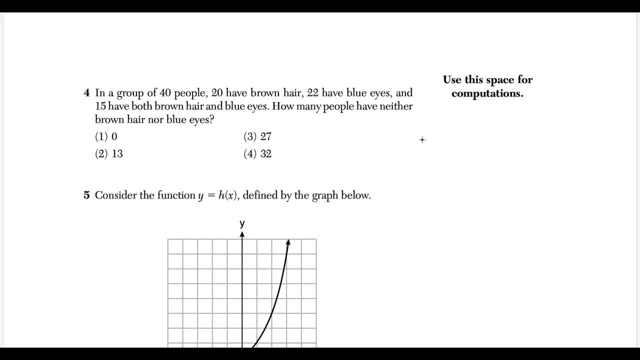 question four: there's a lot going on here, But for questions like this I like to make a Venn diagram. So what we have is we have brown hair, So brown hair is going to go here, And then we have blue eyes, So I'm going to go ahead and just write blue over here. Now I know it's hair versus eyes. 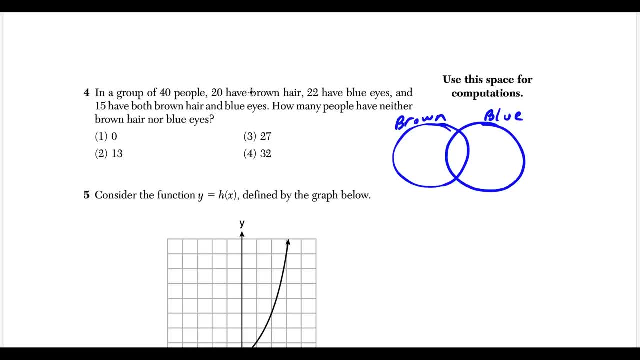 but this should be enough to get the message across. So we have 20 people have brown hair, 22 people have blue eyes and 15 have both. I always like to start with both here, So I'm going to put 15 in the both category. 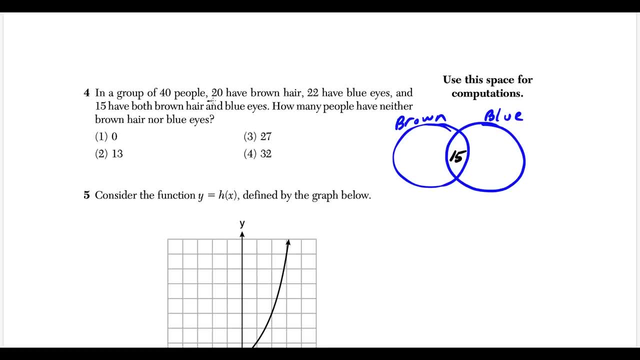 which is where they overlap. So now let's do a little bit of simple math Once again. 20 people have brown hair. So if 20 people have brown hair in total and 15 have both, that means five is going to go here. And now 22 people have blue eyes, that means seven is going to go here. because this: 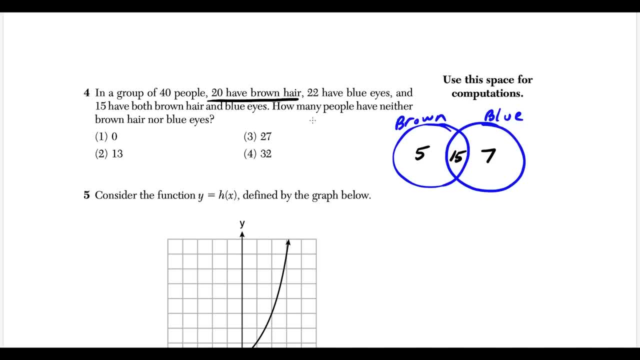 15 plus seven has to equal 22.. So now we want to know how many people have neither brown hair nor blue eyes. So how many people are not in this category here? So if you just add those up, we're going to have five. 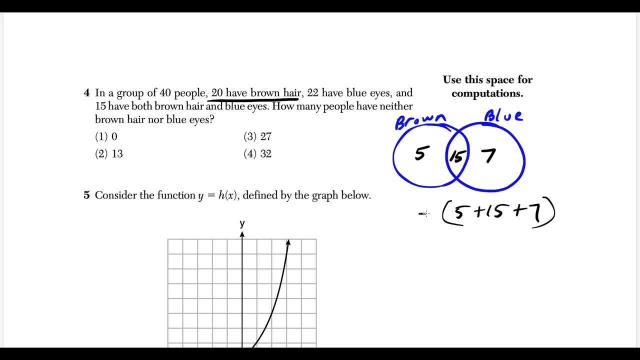 plus 15 plus seven, but this total we're going to subtract from the total amount of people in the group, which is 40. So if you do 40 minus, this is going to work out to 20 plus seven, which is 2740. 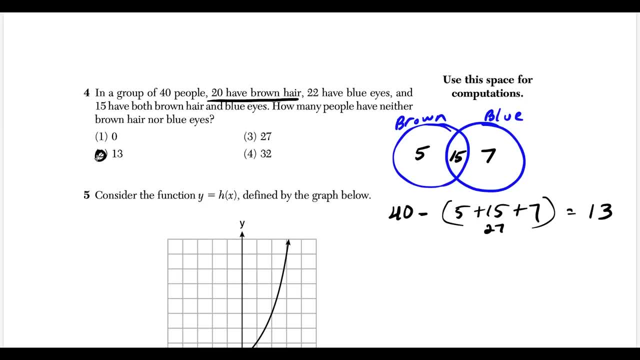 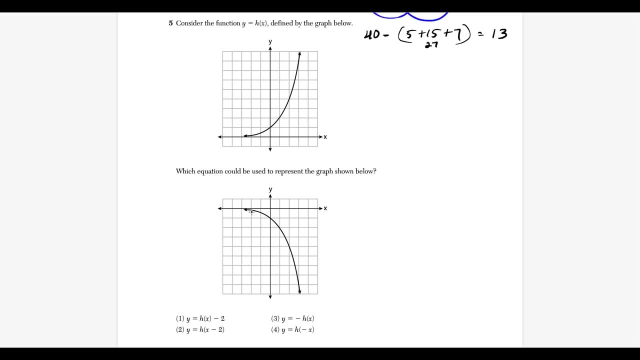 minus 27 is equal to 13.. So this is definitely choice two. For question five, we have a graph of h, of x, And we want to know which equation could be used to represent the graph shown below. So what jumps out at me first is that we have a reflection over the x axis to get from this graph. 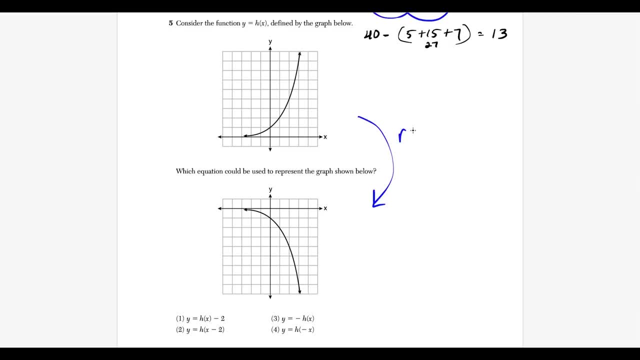 to this graphic, because you could see that this is a mirror image over the x axis. So once again we have a reflection, a reflection in the x axis. Now what this tells me is we need to think about what is the formula for reflecting a function over the x axis And just know if you're. 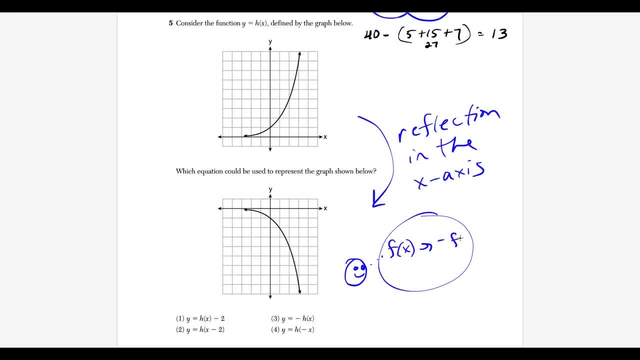 sending f of x, x-axis. you just throw a minus in front and this will send it over the x-axis. If, let's say, we wanted to send the function over the y-axis, Well, for a y-axis transformation, what you do is you. 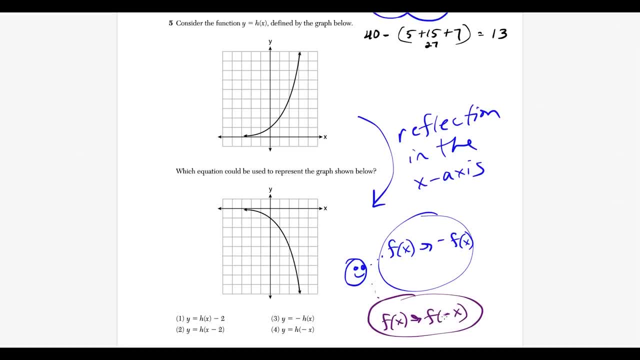 replace the x with minus x, like this. So, once again, if you send, if you replace x with minus x, that will reflect a function of the y-axis. So now we're just looking for one where we have this specific transformation for reflecting in the x-axis. And if we look at the answer choices, 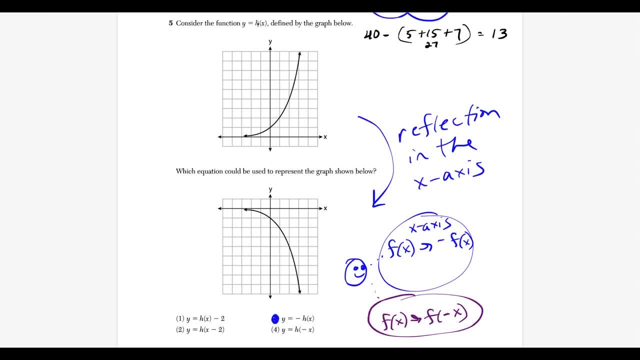 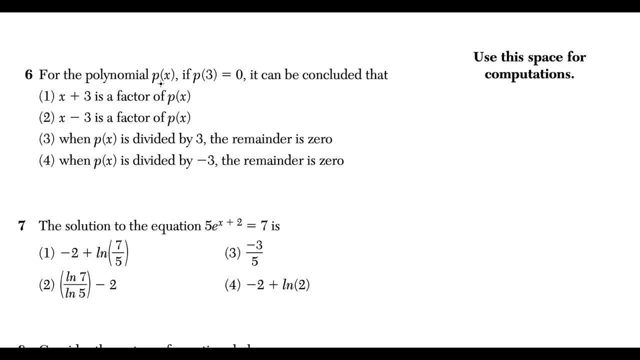 here this is going to match up with choice three, because if we're starting with h of x, throwing a minus in front, we'll just flip it over the x-axis. So question six is a nice conceptual question. We have a polynomial p of x and we're told if p of three is equal to zero, 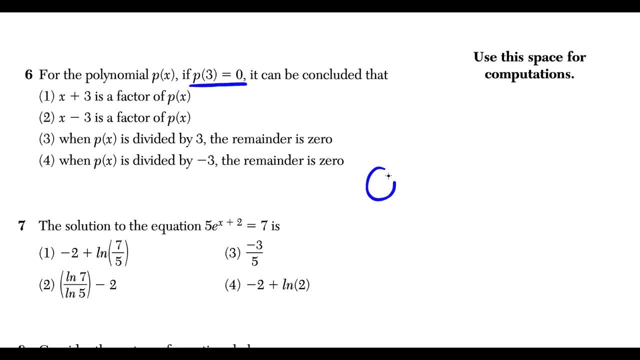 what conclusion can we draw from this? And what jumps into my mind immediately is that when we are told that a specific value of x makes our function equal to zero, this tells us that x equals three is a root. So if x equals three is a root, 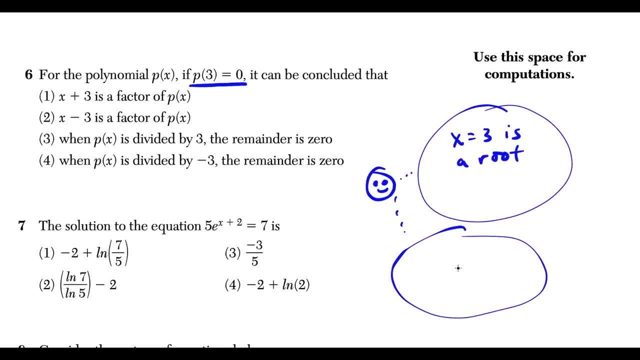 we have to think about the function of x. So if x equals three is a root, we have to think about the function of x. So if x equals three is a root, we have to think about the. how do we get to that point where our solution is x equals three? Well, what we have right before. 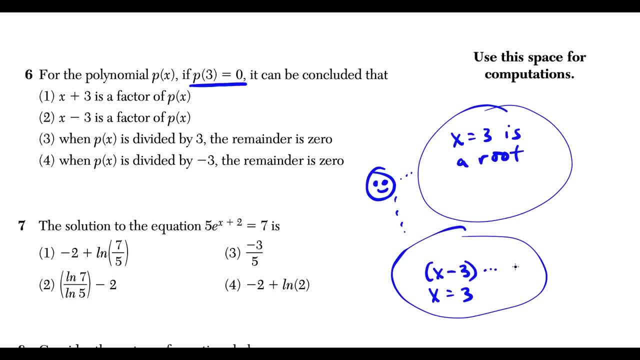 it we would have something like x minus three times. maybe a whole bunch of stuff is equal to zero because we take the factors, we set them equal to zero and we solve for x. So we're kind of working backwards here. If x equals three is a root, this tells us that x minus three is going. 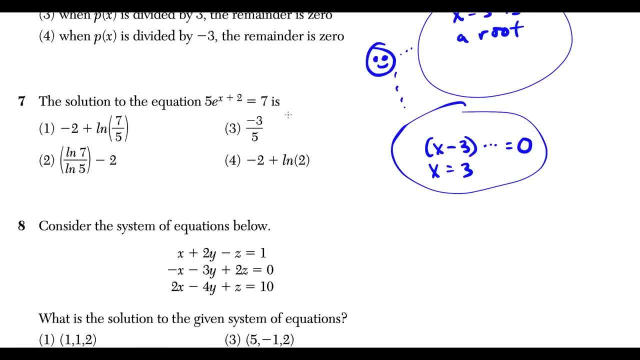 to be a factor of the function p of x. Question seven: I'll show the work in this space over here, and we want to know the solution. So the first thing that jumps out at me is that I would just divide both sides by five, like this: 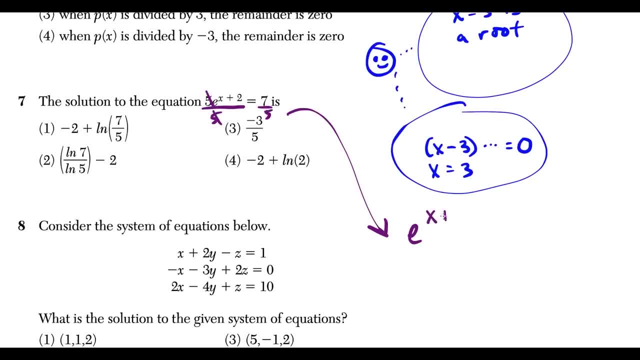 And now five over five cancels and we're going to have e to the x plus two is equal to seven fifths. And now, from this step, we have to know what is the opposite of e. Well, the inverse function for e is going to be natural log. So we're just going to do natural log of both sides. 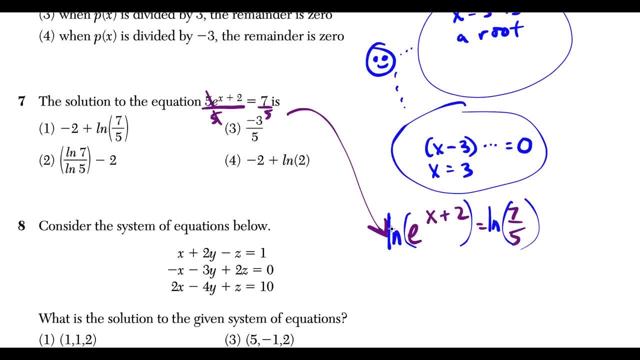 like this. So we have the natural log of the right side and the left side, And now natural log and e cancel out, And this leaves us with x plus two is equal to natural log of seven over five. And now to solve for x, just subtract two. So you have x equals natural log of seven fifths. 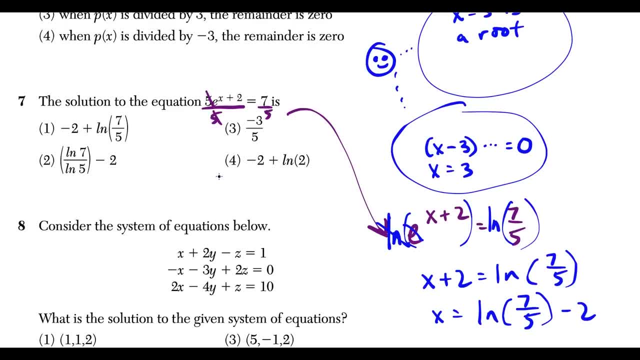 And then we just tack on the minus two And this is going to work out to choice one. The only difference here is that the minus two is in front. So minus two plus natural log is the same thing as natural log minus two. So definitely choice one. Now for question eight. we could do this by hand. 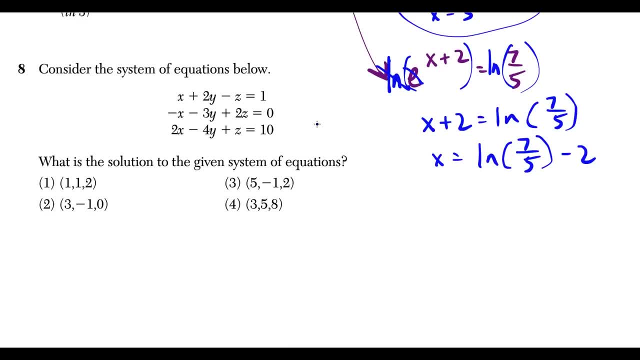 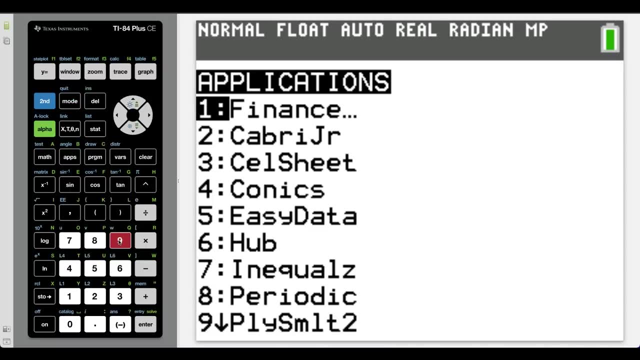 but we are allowed to use a calculator for the region, So let's just switch over to the calculator view. So for this question we could go to apps and number nine, I believe. that stands for polynomial simultaneous And there's a two in front. But what we're going to do is we're going to do a. 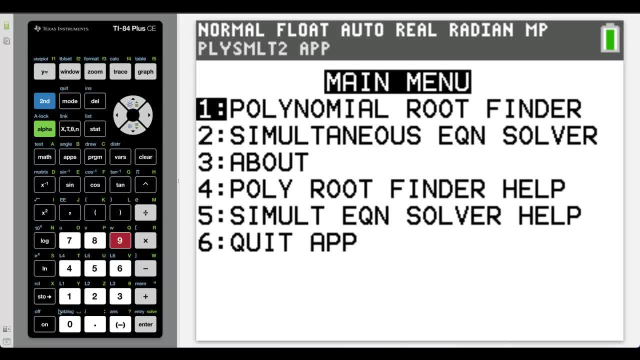 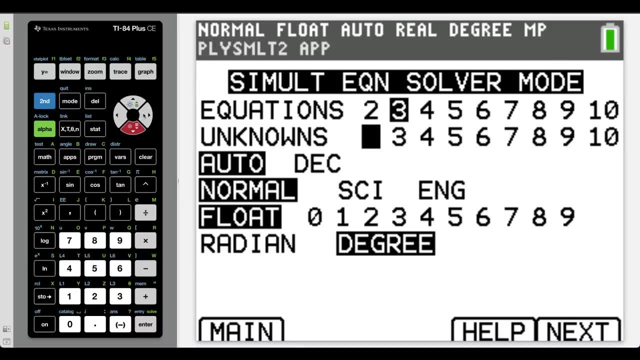 simultaneous equation solver. So we're going to go with number two here, And for this one we're going to have three equations And we have three unknown variables: there's an, x, y and z. So we just have to make sure that we set this up first, And now to hit next, we're going to press the. 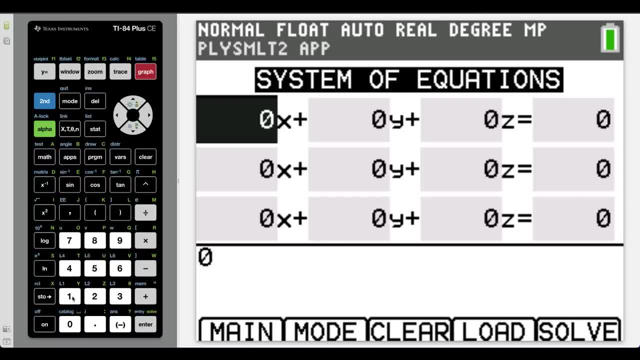 graph button And now, once we go here, we're just typing in: it was one x And then we had plus two times y. So we're just writing in the coefficient two And then we have minus two times y And then minus z. So I could put a minus here And then after this I could put a one in front of the z. 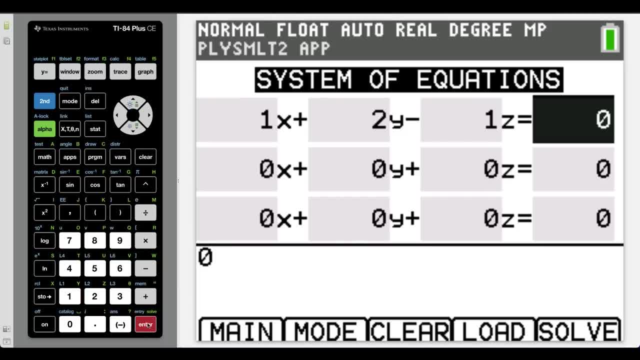 Another way of doing it is you could say plus negative one times z. But either way, this is going to work out fine. And this was equal to one. So now we just repeat this process, But we write in the coefficients: we had negative x, So I'm just going to put the invalid input. So let's. 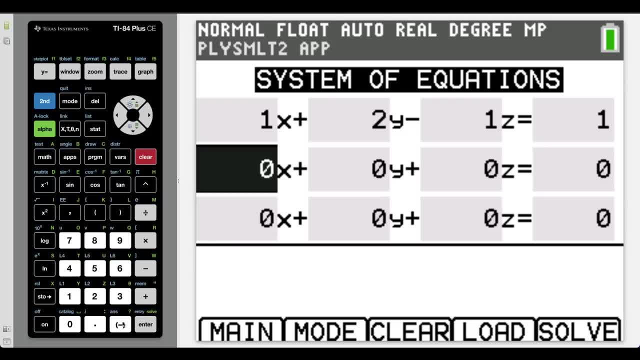 just make sure. we're going to put a negative one in front. So let's clear this out: we're going to do negative one And there we go. So you have negative one x, and then we have minus three times z, And then we have plus two times z. So plus two times z, like this, And now this is equal. 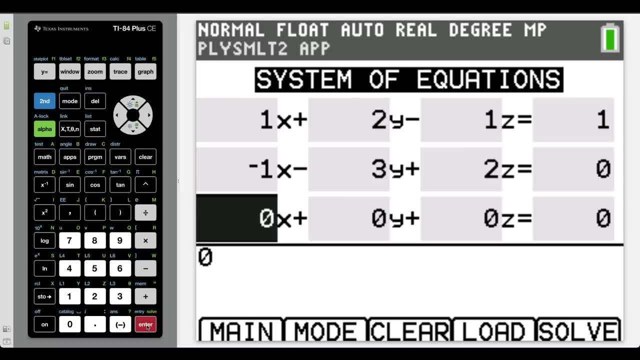 to zero. So that part we just hit enter And we'll move on to the next row. here we have two x, and then we're going to have minus four times y And then we have plus one z, So plus one times z. 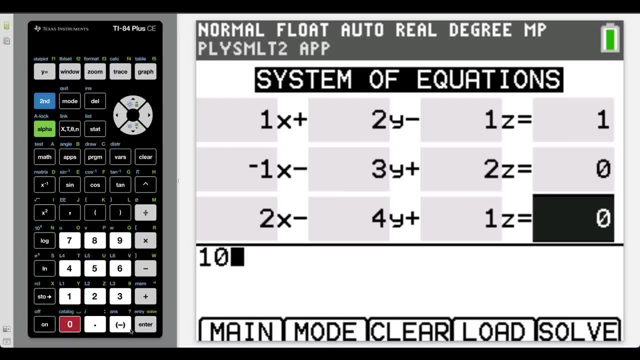 And this one is equal to 10.. So once we type everything in, this is just like a quick process here- we just type everything in Now, we just press graph button, And then we have minus three times z, And then we have minus four times z, And then we have minus three times z, And then we have. 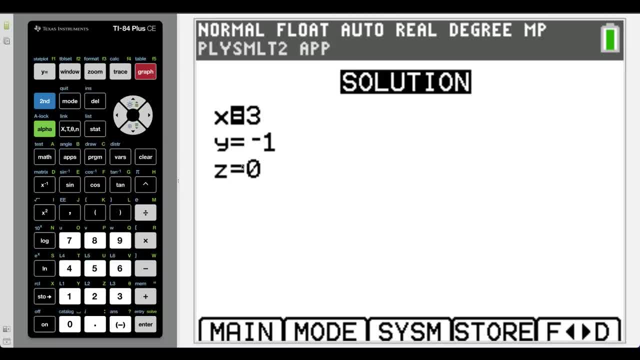 minus four times z, And then we have minus four times z, And then we have minus one times z And our solution is: x equals three, y equals negative, one z equals zero. So number eight: we have: x equals three, y equals negative, one z equals zero is choice two. Our question nine. there's a lot. 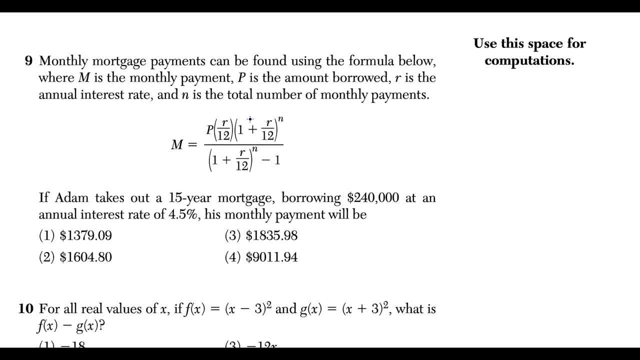 going on. we have this massive formula here for mortgage payments, where capital M is the monthly payment, P is the amount borrowed, and we have: R is the annual interest rate and N is the total number of monthly payments. So now I would just define variables and then type the rest of this. 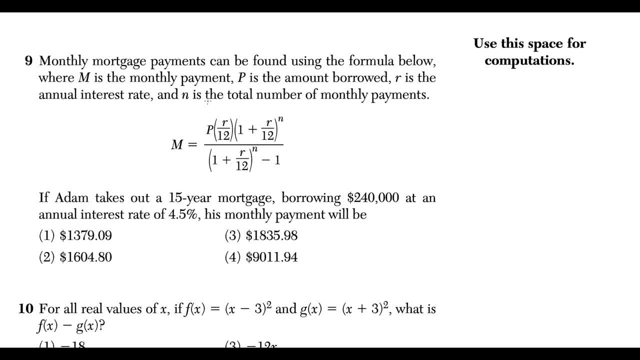 in a calculator. So Adam is taking out a 15 year mortgage, So we're going to type in the rest of this. So if N is the total number of monthly payments, we have to think here that N is going to be equal to. there's 15 years to pay this mortgage and there's 12 months in a year. So 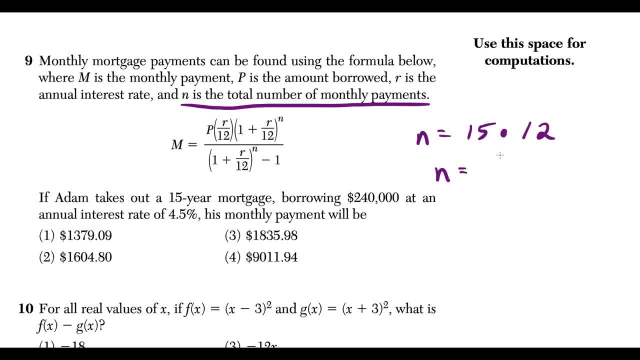 we're going to be making 15 times 12 payments. So this tells us here, if we work this out, that N is equal to 180.. And now, after this, what we have is the principal amount. how much are we borrowing? 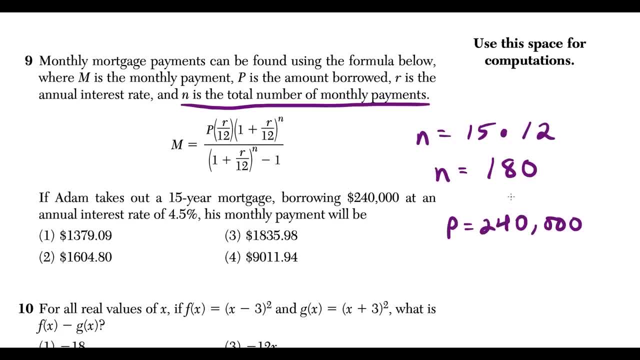 We're borrowing- or Adam's borrowing- 240,000.. So that's the value for P And now the R value here. 4.5% of the monthly payments. So that's the value for P And now the R value here. 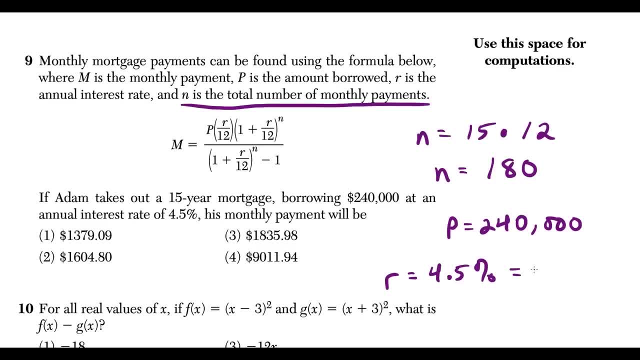 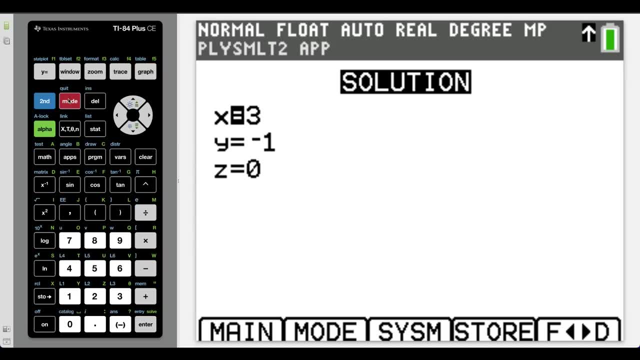 we have to express as a decimal. So if you just do 4.5 divided by 100, you're going to get 0.045, like this. So now the rest. we just type this into the calculator. So if we go back to the 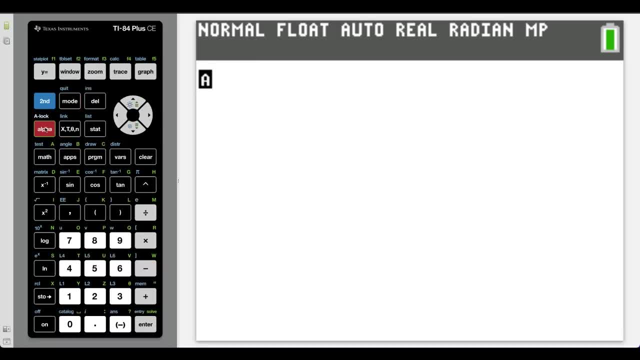 main screen here, so we're just going to press second mode to quit this. I highly recommend, when you're typing in fractions, to write alpha, y equals enter, and it'll pull up a blank fraction like this: So we had capital P, which was 240,000.. So that's our first input value here. And then we had 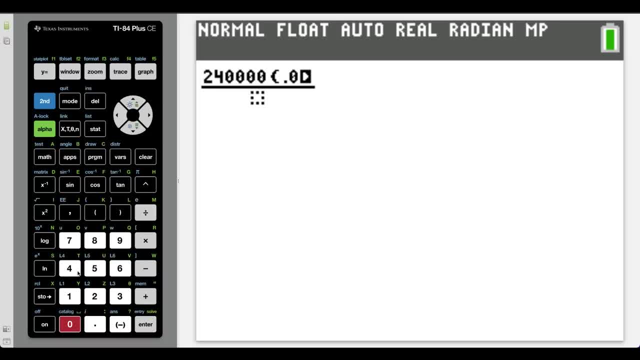 R divided by 12.. So remember, R was 0.05.. So that's our first input value here. And then we had 0.045.. So we're dividing that by 12.. And then next we have one plus. So we have one plus the. 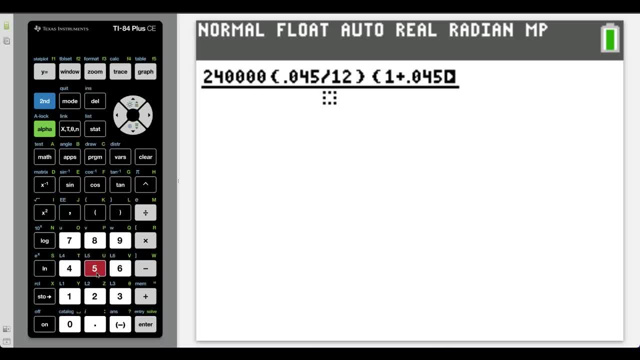 interest rate once again is 0.045.. And then we're dividing by 12.. And we're raising this to the n power. But remember, n was equal to 15 times 12, or 180.. So we're just going to tack on a 180. 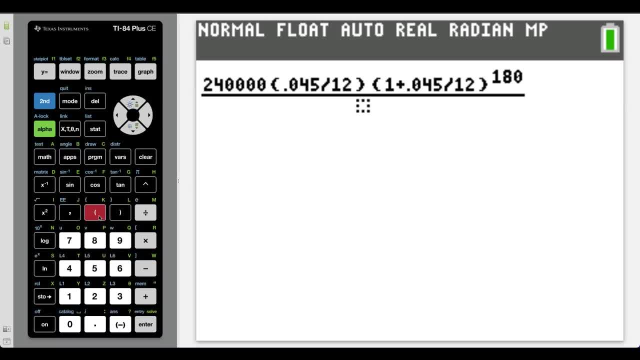 here And the denominator was one plus. So now we just write it: we have one plus the interest rate. So still 0.045 divided by 12.. And this is being raised to the n power. n is still 180.. And then 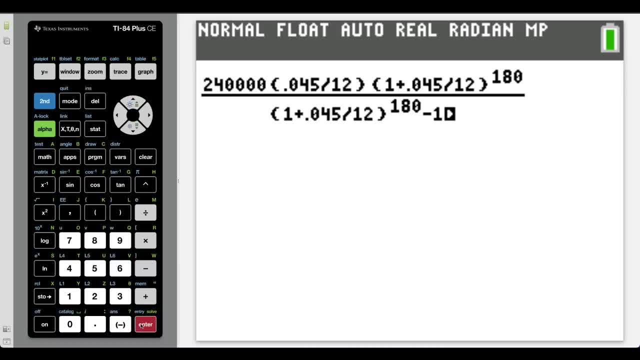 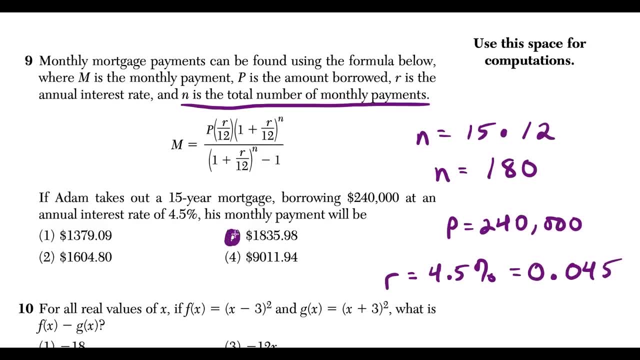 we're tacking on a minus one at the end of all this. So our monthly payment is going to be 1835 and 98 cents. So number nine is choice three. So question 10, we have f of x and g of x And we 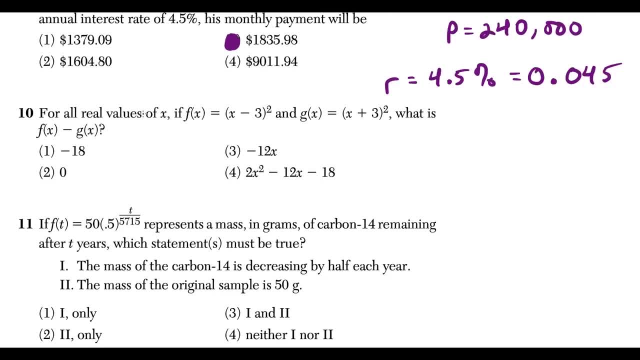 want to know what is f of x minus g of x, And this is for all values x. So for this one here I would just plug in: And we have to know: x minus three squared is the same thing as doing x minus three times x minus. 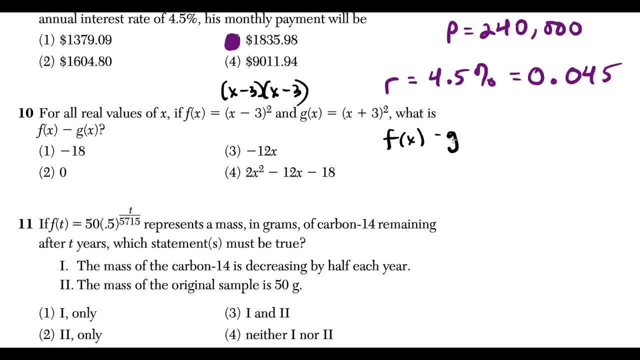 three. So what I have here, if I want to find f of x minus g of x, f of x, we just expand this here is going to be x squared. we would have minus three x. So we have x squared minus three x minus. 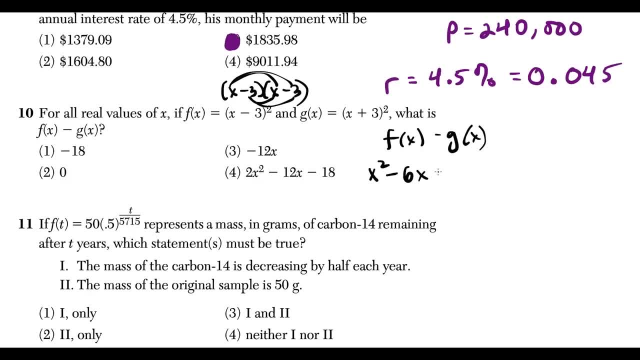 three x, which would give us minus six x. And then minus three times minus three gives us nine, And now I have minus. and we have to watch out for this trap here. When you're subtracting a polynomial, please make sure to put it in parentheses. 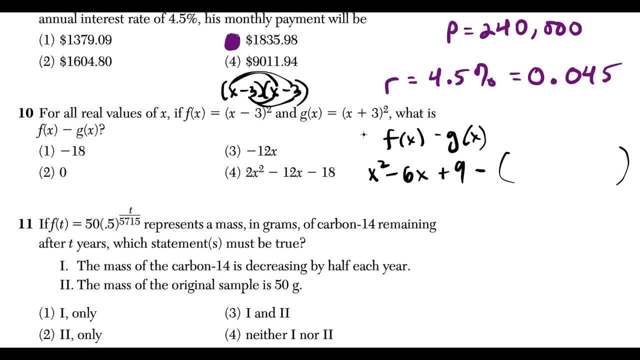 You only subtract the first term. that's just going to throw off the whole question. So now g of x is equal to x plus three times x plus three. So if we expand this, we have x times x, is x squared? then we would have plus three x plus three x, which gives us plus six x, And then three times three at. 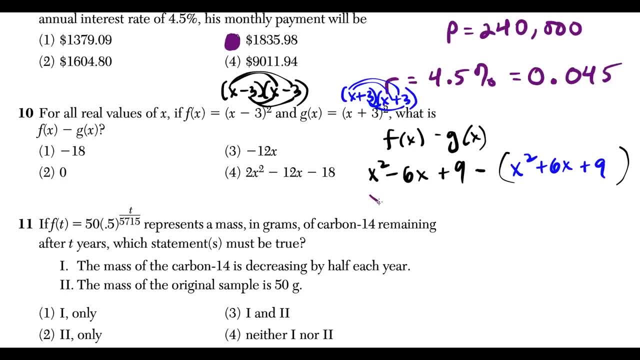 the end is nine. So that brings us here And now. if we work this out, this is x squared minus six, x plus nine, And if we distribute the negative we get minus x squared. then we have to distribute the negative here: we get minus six, x and we get minus nine. 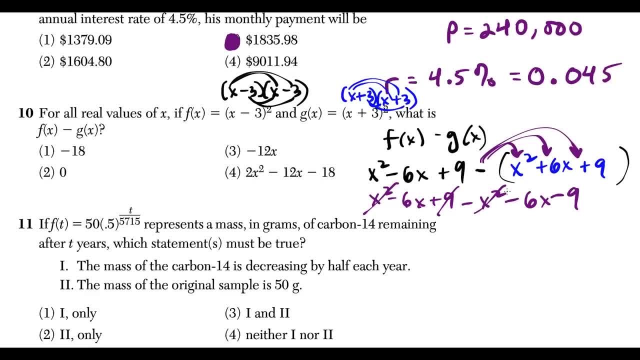 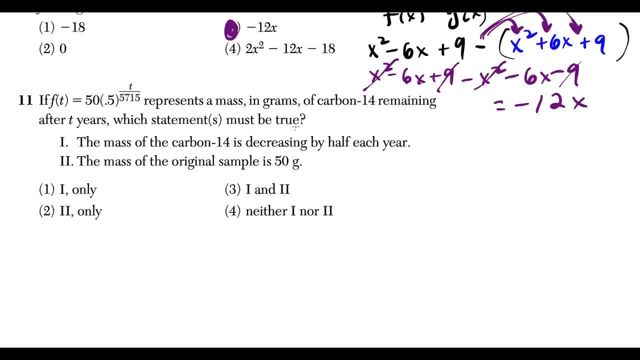 So almost everything cancels out. the x squares go, and then nine minus nine cancels, but minus six x minus six x gives us minus 12 x. So this is definitely choice three. Question 11, we have f of t And this represents the mass in grams of carbon 14 remaining after two years, And this is 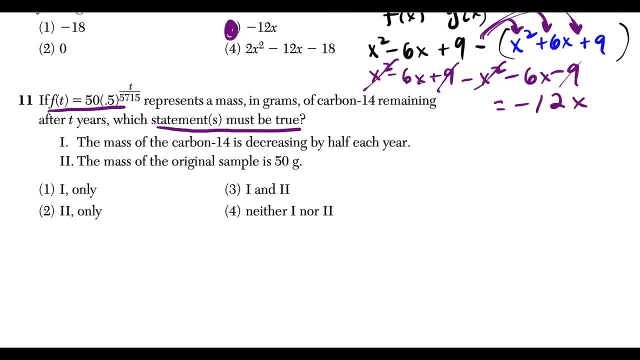 what we want to know, which statements must be true. So if we go through these one by one, for Roman numeral one we have, the mass of carbon 14 is decreasing by half each year. Well, just know that t is modeled with years. So if the mass is decreasing by half each year, that means if we were, 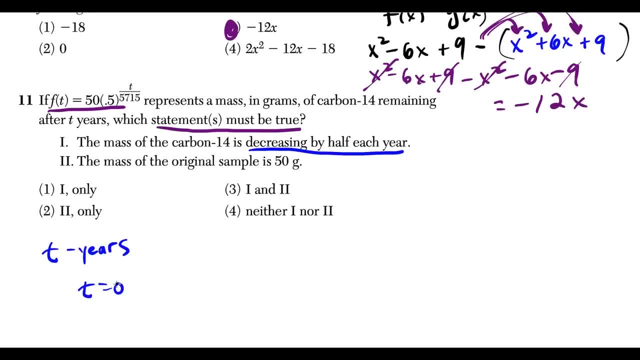 to plug in, let's say t equals zero, t equals one, that this thing would just keep getting chopped in half every time we go up by a year. But the problem with that is that we have t divided by 5,715.. So 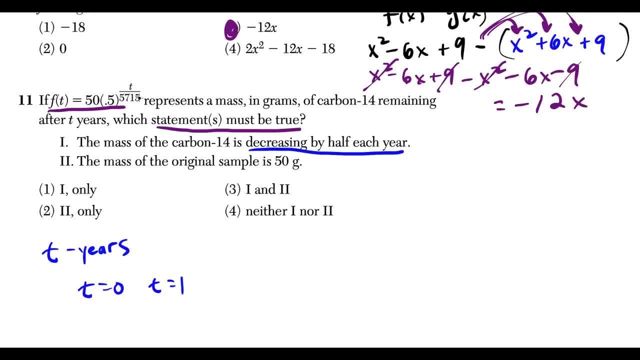 this would actually take 5,715 years to cut things in half. So Roman numeral one is out. for that reason, Because, once again, if we look at this, if we have 50 times 0.5, to, let's say, the 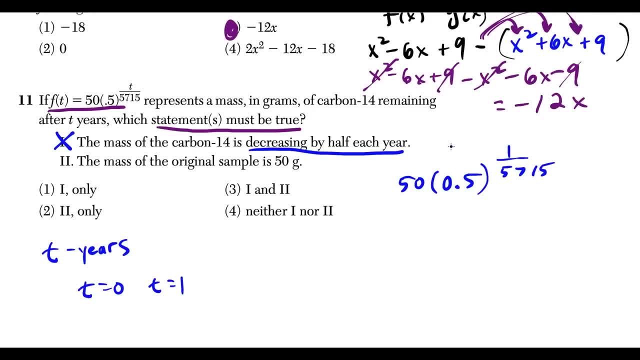 one over 5,715, this would be: t equals one. if we were to go forward one more year, we would have 50 times 0.5 to the two over 5,715.. So if you were to compare these values here, this new value is not. 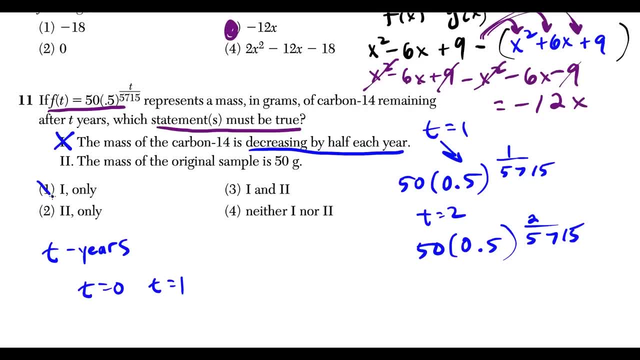 going to be half of the original. So once again, that's why Roman numeral one is out. So this is two and four. So now we have to fact check Roman numeral two And if we go forward with this one, the mass of the original sample is 50 grams. And to check this one, the mass of the original refers. 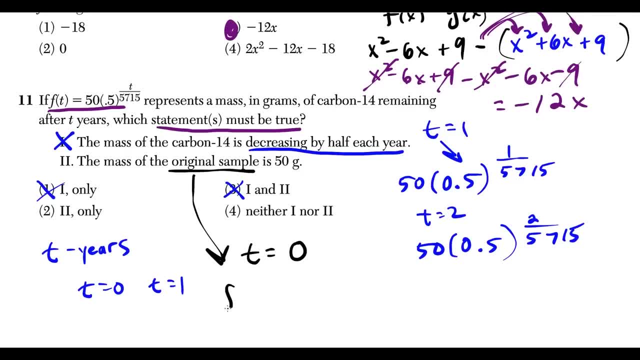 to time t equals zero And if you were to plug in t equals zero, you'd have f of zero equals and we'd have 50 times 0.5 to the zero over 5,715 would give us to the zero power, And then 0.5. 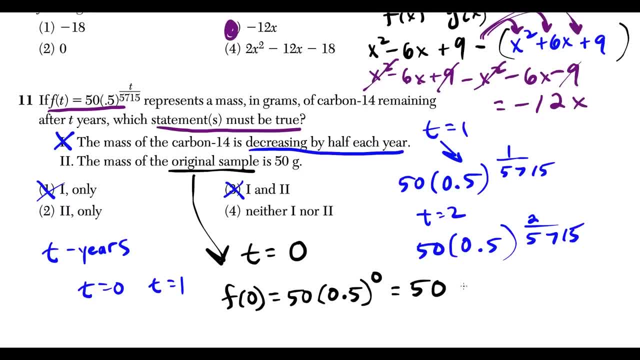 to the zero is equal to one, So this would just be equal to 50. And the mass is grams. And notice what they told us here, that they told us the mass of the original sample is 50 grams And this worked out to 50. So Roman numeral two is true, which means choice two. 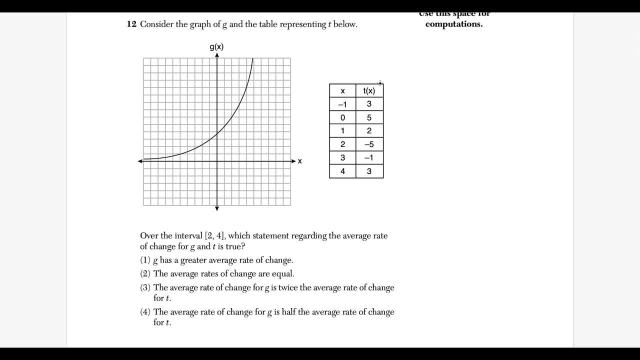 is our answer. So question 12, we have a graph of g and a table for t of x, And we're talking about the interval from two to four. we want to know which statements regarding the average rate of change for g and t is true. So the first thing that's jumping into my head for this is when I 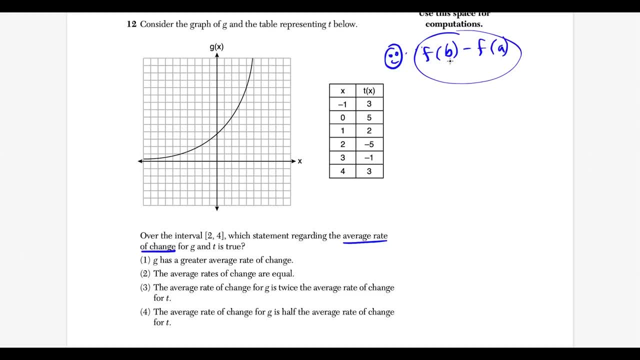 hear average rate of change, I automatically think of this formula: f of b minus f of a over b minus a. So that's where my attention shifts. And since we're going from two to four, I'm going to look at this graph here. at x equals two, I just count up. we're going. 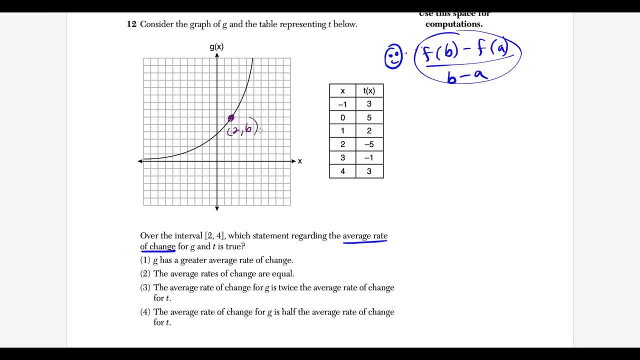 up 123456.. So this is the point two. six, And if we go out to four, we're going over two more. we're going up 12345678910.. So this is the point 410.. So what I would do is I would find the average. 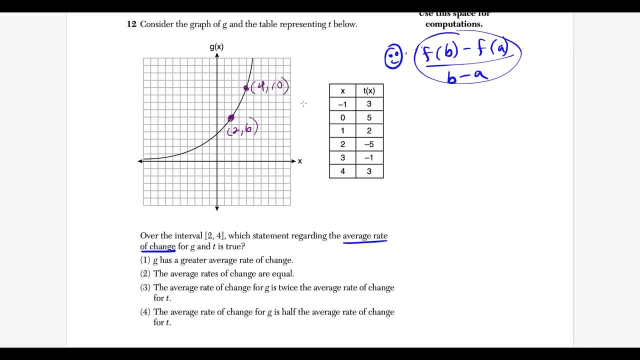 rate of change for both of these. So for g of x, the average rate of change is going to be: we could say: here is 10 minus six. So now we're just finding the slope over four minus two, And then we get four divided by two, which is two. So this is once again for g of x. on the interval, 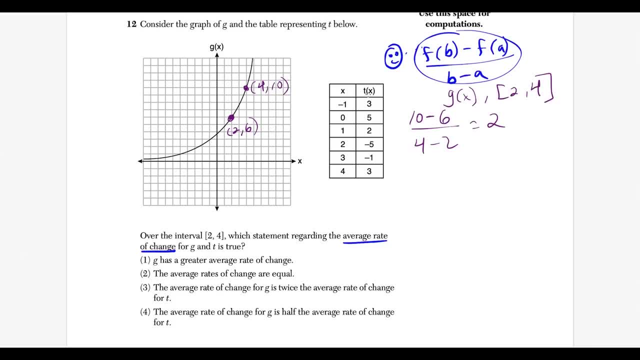 from two to four. But now, if we find the average rate of change for t of x, this will be a little bit easier, Because for this one what we're doing is t of four minus t of two over four minus two. 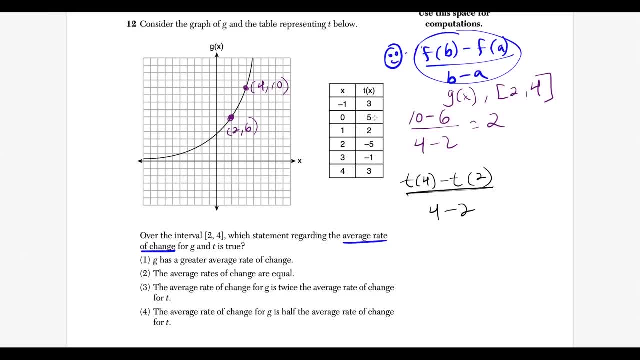 And for this one we have a table, So we don't have to rely on our ability to count. So t of four minus three, So this is equal to three minus. and then we have: t of two is negative five, So we have. 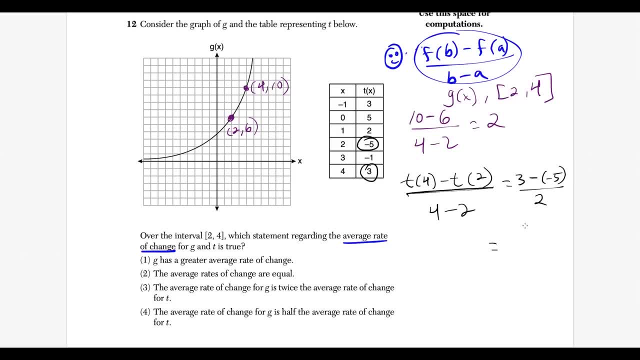 three minus negative five divided by two, And this gives us eight divided by two, which is equal to four. So the first observation that I make here is that t of x has a greater average rate of change than g of x. So if we look here, g has a greater. this is not true. they are not equal. the average. 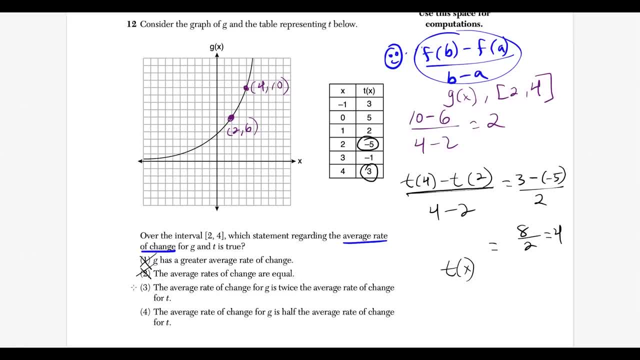 rate of change for g is twice the average rate of change for t is not true, But here's the one: the average rate of change for g of x is half the average rate of change for t of x, because this is two and that's definitely half of four. So choice four is our answer. So for question 13,, 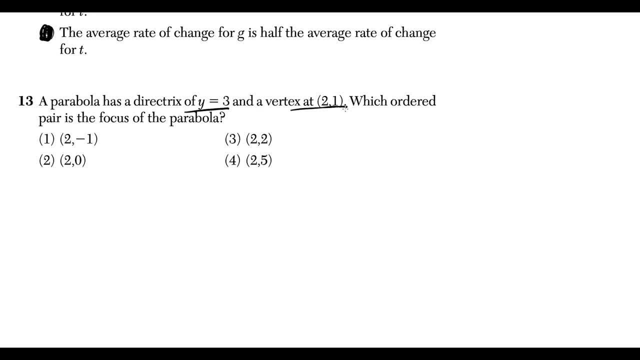 we have the directrix, is the line y equals three, and we have the vertex of our parabola And we want to know where is the focus of the parabola. So for this question, you could know a bunch of formulas for this, But honestly, I can never remember formulas, So I have to think about the 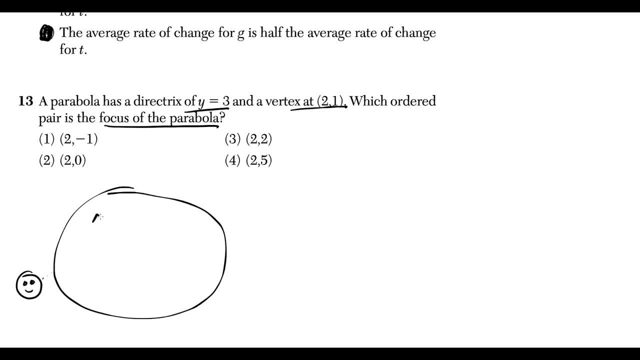 concept involved, And what I know about a parabola is that if it looks like this, if it's smiling at us, we have a focus here. So this is our focus, And then the directrix is right under it, Because the concept is that a parabola is the same distance. any point on this parabola is the same. 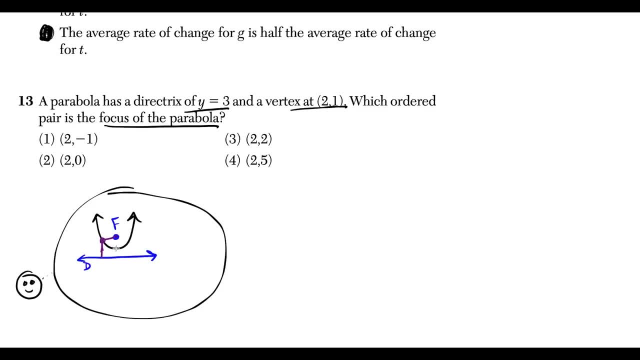 distance away from the focus as it is from the directrix, like this, And if we're using the vertex, it's a straight run. like this: the distance from the focus to the parabola is equal to the distance from the parabola to this line, the directrix. But the other way this could work. 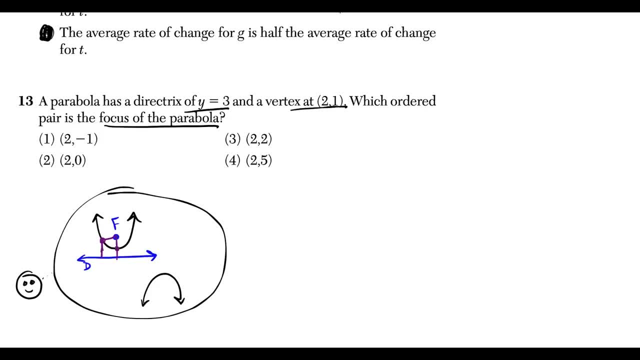 out is we could have a parabola that's frowning at us. We would have the line, the directrix, going above, like this, and the focus would be underneath, like this. And once again, it's still upholding that idea that any point on this parabola, the distance, 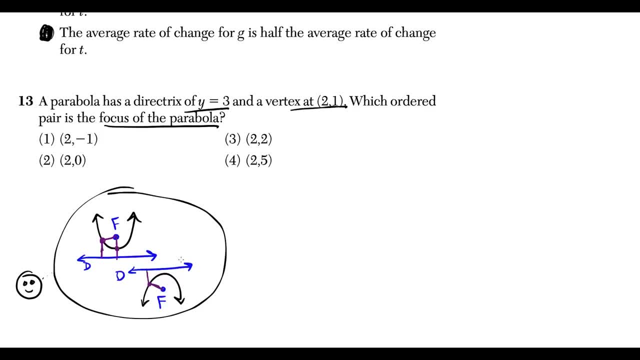 from here to the directrix is equal to the distance from here to the focus. A lot of talking for that part, But now we go ahead and draw this out. They told us the equation for the directrix and they said it's: the line y equals three. So if I go up here, one, two, three. 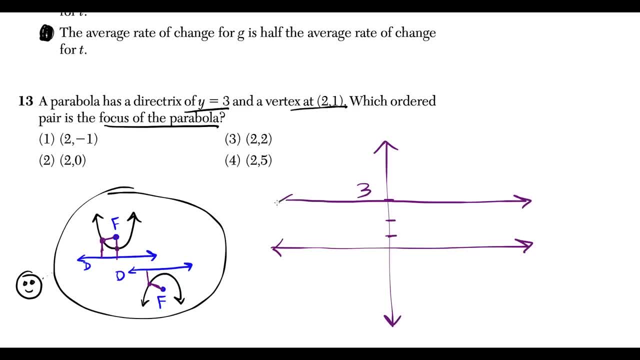 so our line is going like this. So this is the line. y equals three. The next thing we were told is the vertex, and the vertex is at the point two, one. So that's going to be over here And notice, this is the second case where the directrix is above the vertex. So this is the once again. 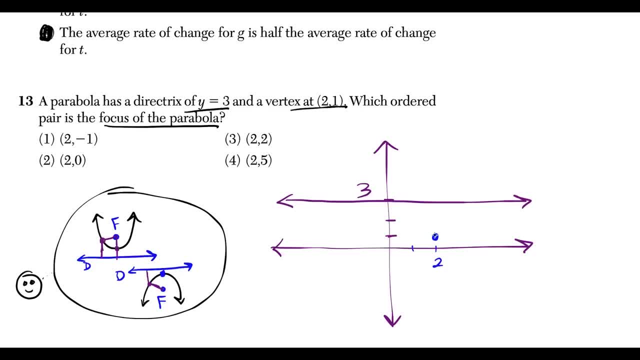 the vertex, referring to the turning point of the parabola. So that means our parabola is going to be opening this way And remember the concept that the distance from the directrix is equal to the parabola is equal to the distance from the parabola to the vertex. I'm sorry, from the 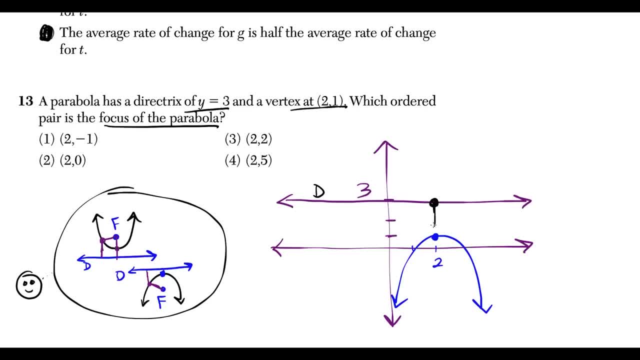 parabola to the focus. So this distance, here we just have to count. This is the point two, three, and the vertex is at the point two, one. So how far away are these points? you could just count. we're going up one, two. So there's the distance. So the focus has to be two units away from the 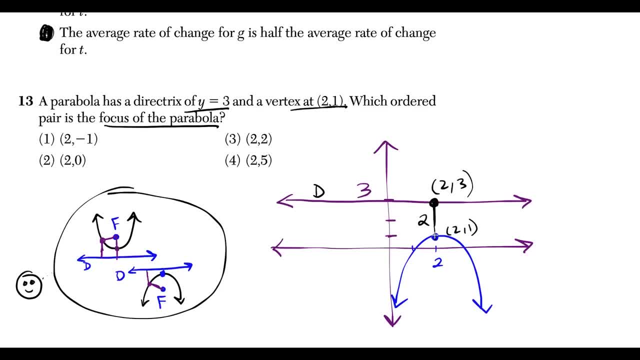 vertex. So that means we would go down to from the vertex. we're going down one, two like this, And that's where our focus is. But now we just have to assign a coordinate here, Since we went down two units. from a y value of one, we're going down to negative one And this: 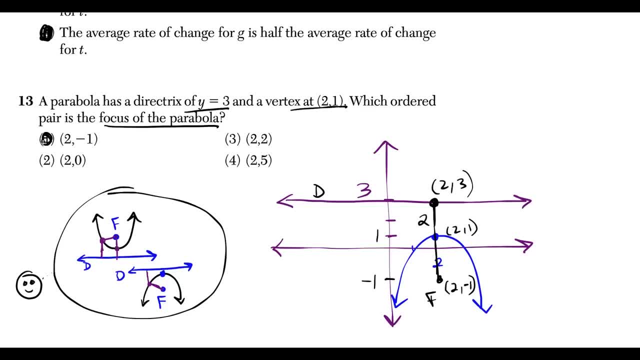 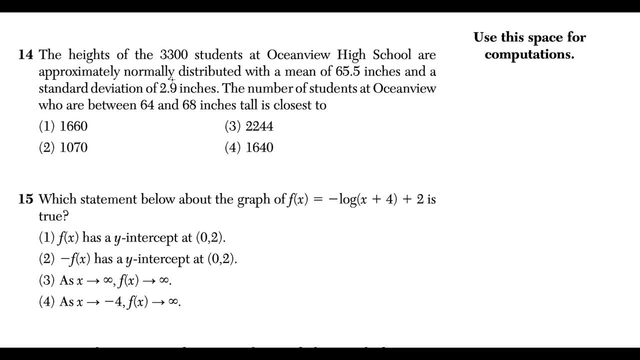 location is two, negative one, which would correspond to choice one. Alright, question 14, not to be negative here, But this is one of my least favorite questions I've encountered in a long time, because I like when you get something exact. But we have the heights of 3300 students at. 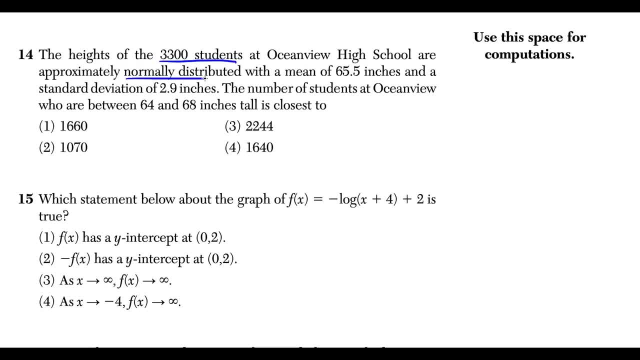 this high school are approximately normally distributed within a mean of 65.5.. And we have a standard deviation of 2.9.. And we want to get a standard deviation of 2.9.. And we want to get a standard deviation which would be causing the highest number of students, putting on不起 main. 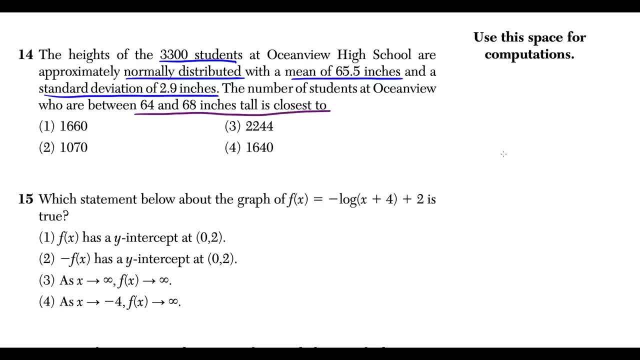 class at one student. So we want to draw a normal bell curve because this is what our average deviation on average is in advertising And would be measured with the average deviation, And we should be making this a standard deviation. Please guide the students by. you know these questions. You. 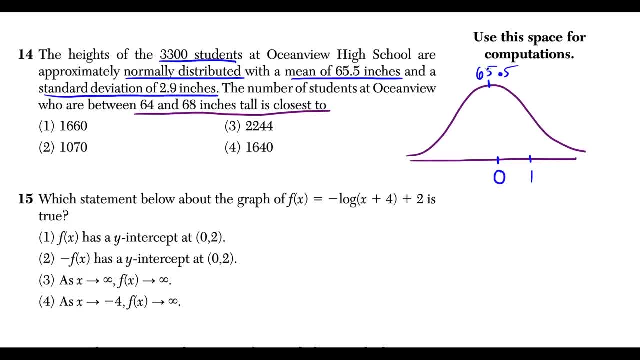 just need to be able to understand the fact that engineer really has a standard deviation. if you had seven degrees less than 30 inches and none of the students are this way to the right, I would add 2.9 to 65.5. you know, I'm going to make this a little bit bigger. 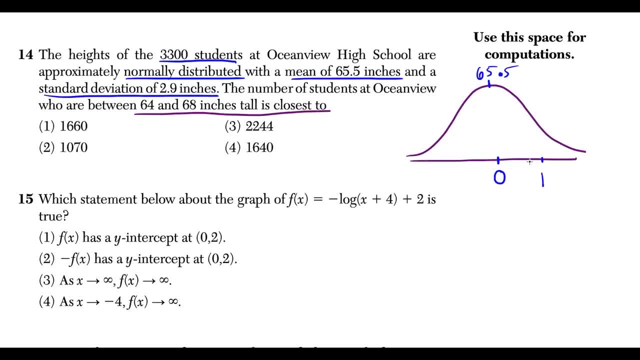 here. so let me just expand this out a little bit so we can really see. so if we were to add 2.9 here, we would get 68.4. so 68.4 would bring us here, and this is pretty close to 68. so I'm going to stop. 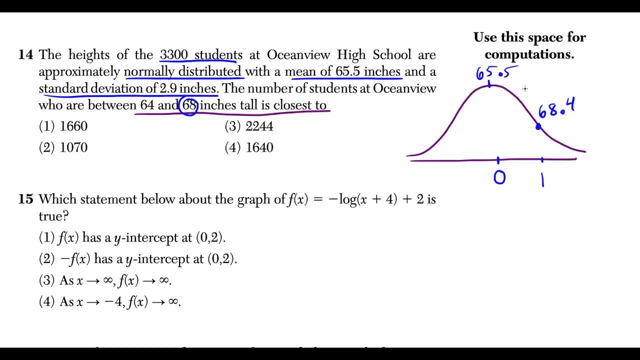 now watch what happens if we subtract 2.9 from the average. if we were to subtract, that would send us one standard deviation back this way, but the problem with that is that it would throw us to 62.6. so once again, if you did 65.5 and you subtracted the standard deviation of 2.9, 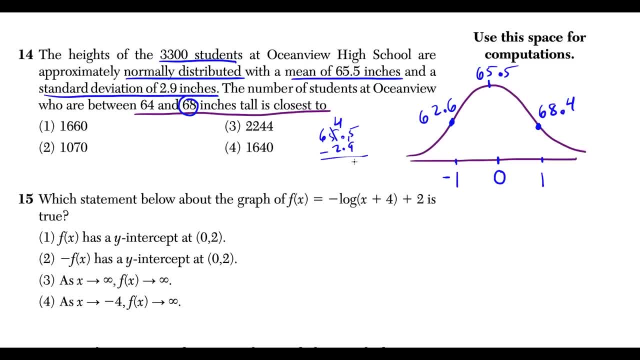 this one here, if we do the math here and work this out, is going to work out to 62.6, and the problem is that that's pretty far away from 64. so then we say, what if we were to take the standard deviation and cut it in half? well, this would be equal to, we would have 1.45. 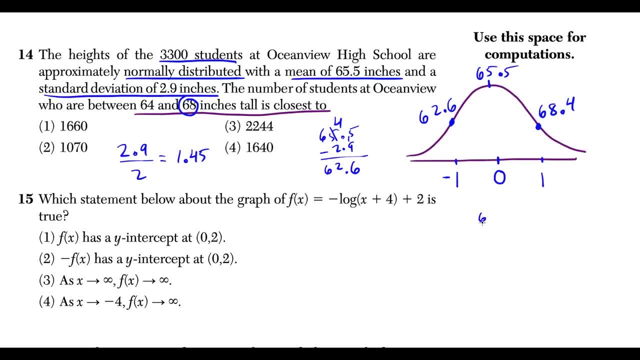 like this, and if we subtract that from 65.5, so we do 65.5 minus 1.45 like this. now, just tack on a zero here. this, we could just work this out- is going to work out to: we would have 64.05, which. 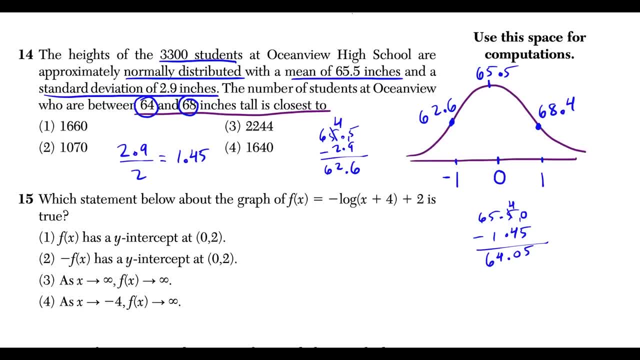 is way, way, way closer to 64. so a little bit of a sneak attack here is that we're going to go half of a steven, half of a standard deviation to the left, which brings us once again to 64.0 five, and we're going to go one full standard deviation to the right. so we're focusing on this. 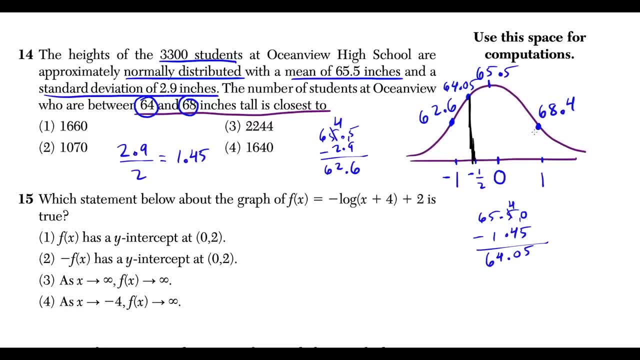 space here. so we're going from here all the way to here. but now one thing that is given to us in- uh, you know, if you have notes on standard deviation- is that this space here is 31.34.1 of all the scores but or, in this case, all of the heights. but if we go half a standard deviation. 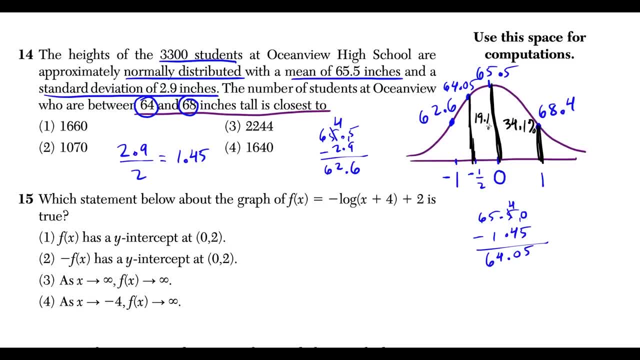 this way. this is not going to work. so we're going to go half a standard deviation this way and we're going to go half a standard deviation this way and we're going to go half a standard deviation and this piece from the half to the full standard deviation is 15. so that's how the 34.1 is made up. 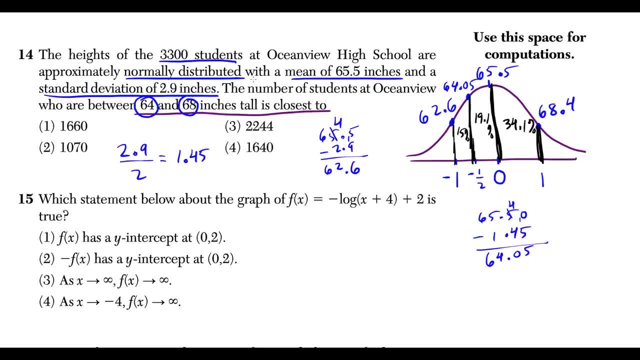 so once again, we're trying to see the number of students between 64 and 68. so that means we're going to be focusing on this slice here. so that means we're going to go half a standard deviation to the left and a full standard deviation to the right, so we have to add these percentages together. 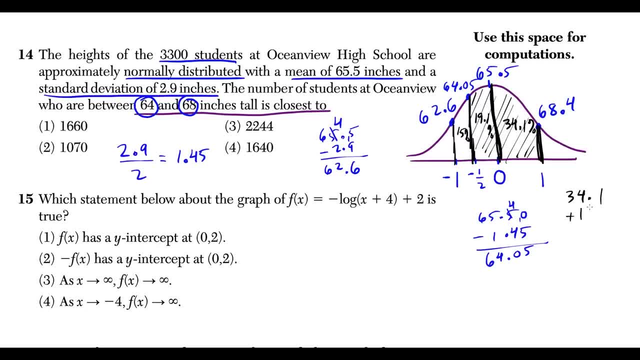 so we're going to do 34.1 plus and then we have- and if we work this out, this is going to work out here to 53.2 percent. so now we're going to take 53.2 percent of 3300, so i have 3300. 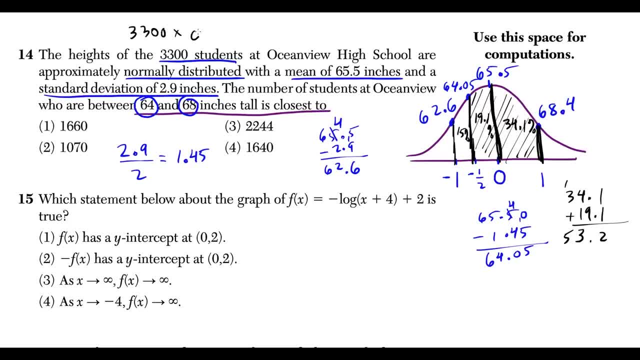 times 53.2 percent, i could express as .532, like this: and if we work this out, this works out to 1755.6. and now if we look at the answer key here, the one that we're closest to, where a little less than a hundred of points is going to be a little bit less than a hundred of points, so we're going to 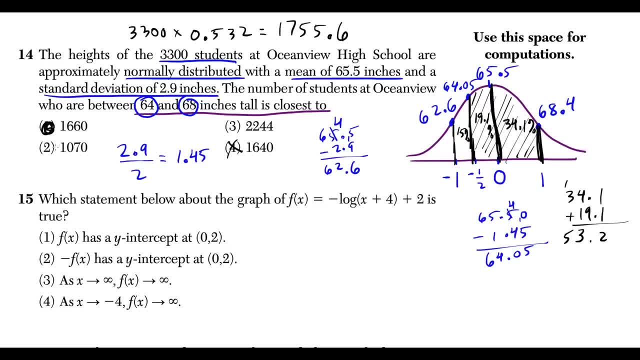 away from choice one, but this one we would be even further away from, and this one and then 2,244 would be us going way, way, way too far forward. So this would be almost 500 units forward from this amount, So this one we're closest to. but the reason I don't like this question is that 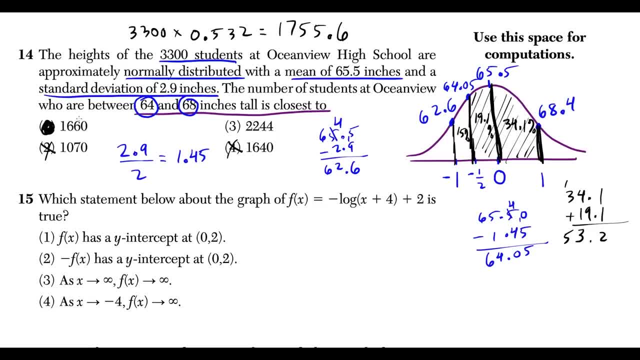 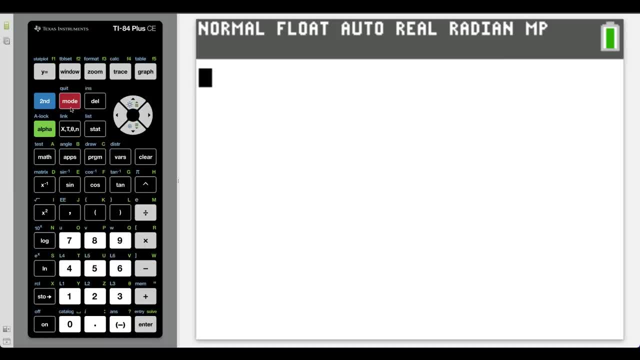 this number is still pretty far from this question. So choice one is our answer. Question 15,. we want to know which statement about f of x is true, and we're going to use the calculator for this. So for this one we'll go to the y equals and we're going to write in the function we have: negative. 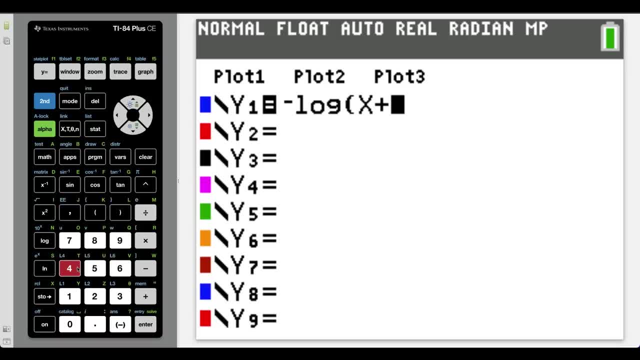 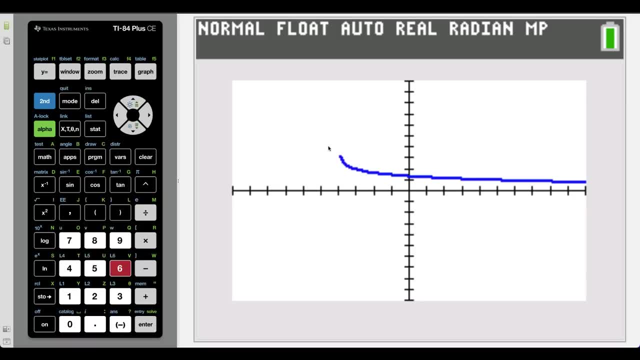 log and then we have x plus 4 inside the parentheses and then close the parentheses and we're going to write plus 2 on the outside. So here's our function: We'll press zoom 6 just to make sure we get a nice picture, and let's go ahead and borrow this. So, while the calculators 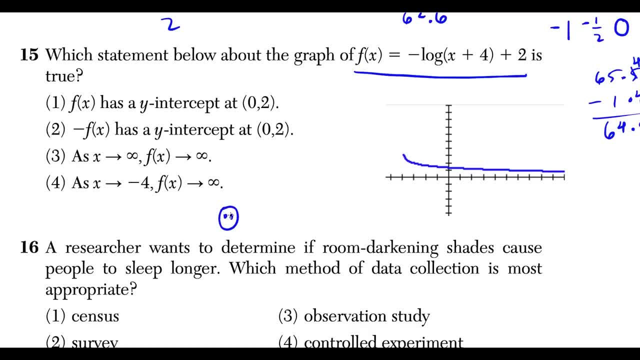 up today are awesome. what I like to think about for questions like this is, I think, about the standard graph of log x, which we can think of as the parent function here. So for just the graph of log x, the point is that we're going to write in the function, so we're going to write in the 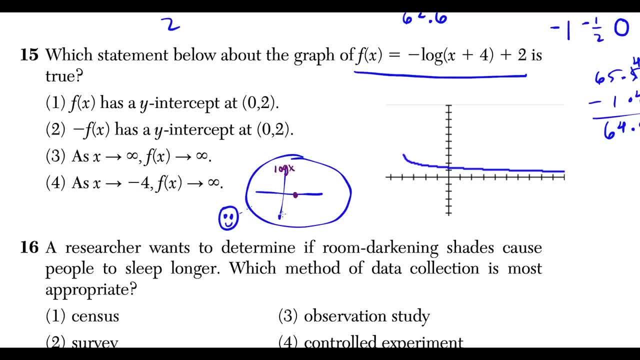 So this was log x. 1, 0 is a point on this graph and it looks something like this. now, what I know about log x is that the y-axis is a vertical asymptote like this, and This graph will go on to infinity like this. so 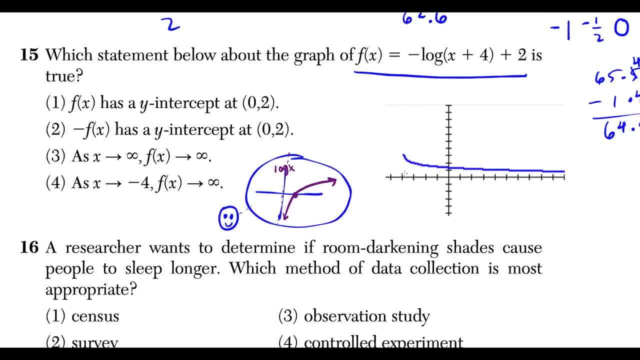 That's one thing I keep in mind, because when you use the calculator, the picture is nice But it doesn't exactly like tell the best story. so looking at this, I could see here, if I go to the left, 1, 2, 3, 4, it. 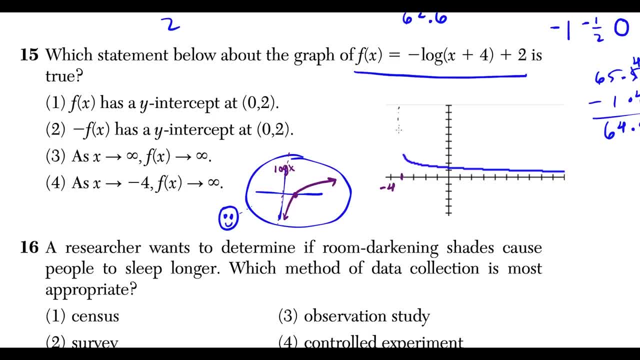 Looks like here, at negative 4, that we have a vertical asymptote. so once again, the calculator is nice, But you have to be able to do part of the thinking here to complete the picture of the calculator. So this calculator will give us a start, but what we have to be able to fill in is that at x equals negative 4, we have a vertical asymptote and 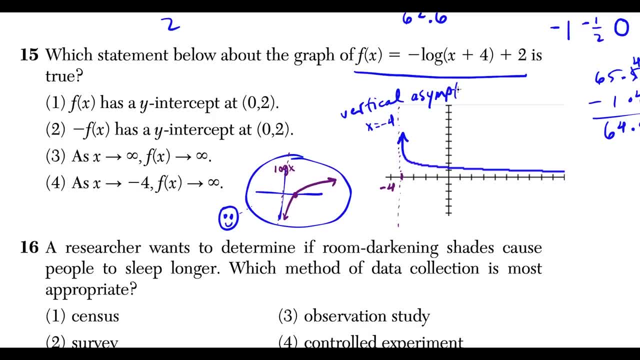 That's going to help us answer this question, because without even looking at the answers here, I'm going to see here that as x approaches negative 4 On the right side, we're going up to positive infinity like this. so this one 15 is looking like choice 4. 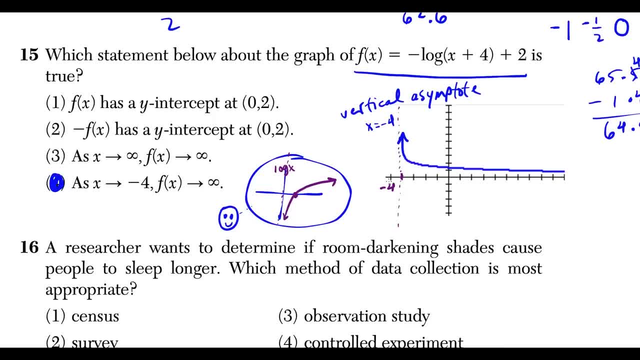 Now, the one lazy detail about this question is that there's nothing going on to the left of negative 4. so what they really are Saying here- if I had to make this a better question- is that x is approaching negative 4 And we're going to say here from the right side, because, once again, 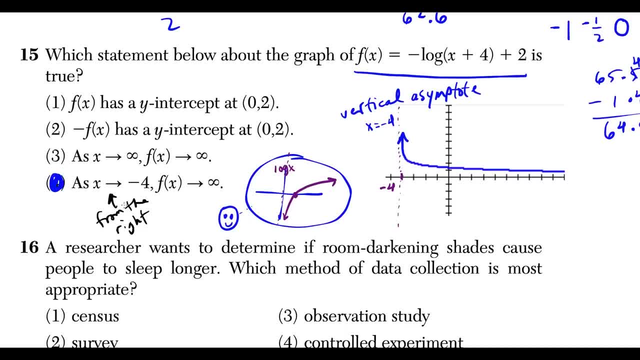 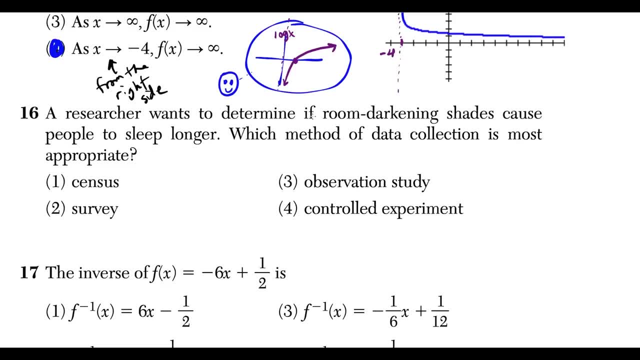 There is no graph on the left side of x equals negative 4, But we're approaching negative 4 from the right side and as we get closer to x equals Negative 4. the graph is going up to infinity. question 16: We have a researcher that wants to determine if room darkening shades. 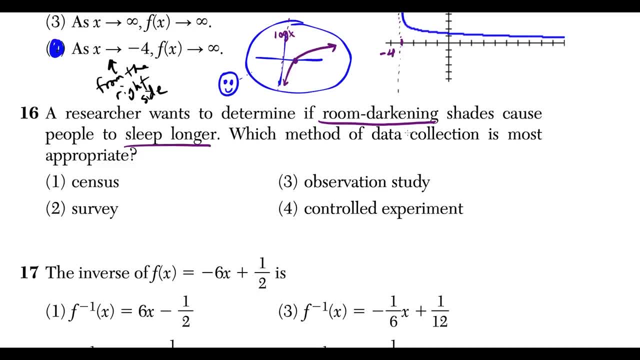 Cause people to sleep longer, and we want to know which method of data collection is most appropriate. So we have a census, a survey, observation study or a controlled experiment. well, in this case, a controlled experiment would work best, because We would put some people in a room without these room darkening shades and some people in a room with the room darkening shades. 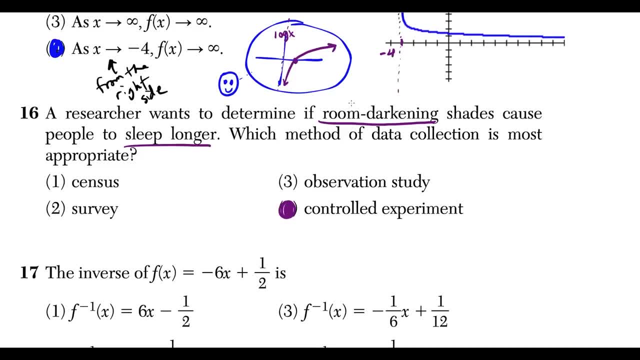 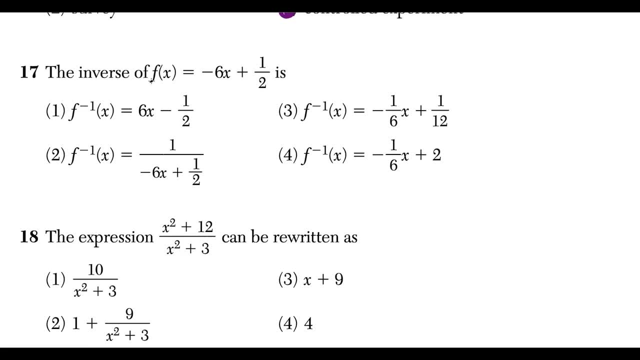 To see if it has any difference On the quality of their sleep, and I'm sure they would select people that have Around roughly the same average amount of hours of sleep each night. But choice 4 is looking like the best. so question 17 is all algebra when we're finding the inverse of a function. 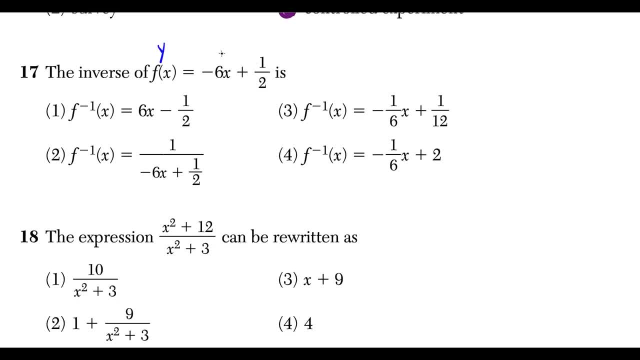 I think of this as y equals this function of x, and when you want to find the inverse, just switch the X's with the Y's and then solve for y. so instead of y equals this, we're gonna have x equals negative 6y Plus a half. so then from here We're solving for y. This is the variable that we want, so we just start doing. 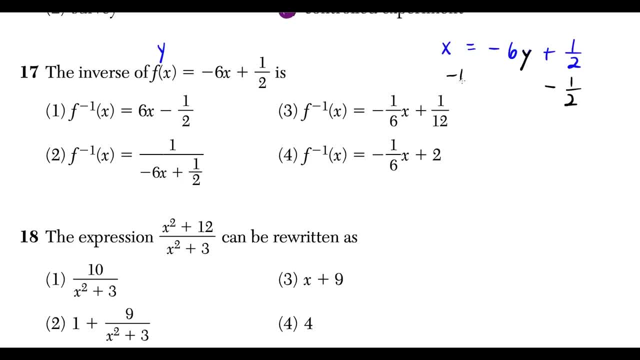 The opposite operation. so we're going to do minus a half on both sides. so we subtract a half and What this is going to give us we're going to have x minus a half is equal to negative 6y, And then from this step, we're going to divide everything by negative 6, so we're going here like this divide. 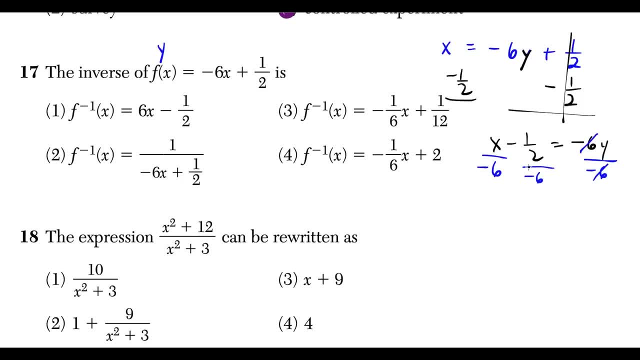 Everything by negative 6, and now we just have to match it to how it's written in the answer key. But now we have y equals and then there's an invisible 1 in front. So I could write this as 1x over negative 6, or I could call it negative 1 over 6. 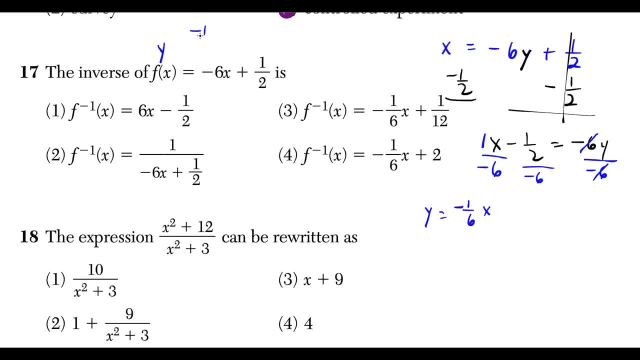 times x and just know, when we do negative 1 over 2 Divided by negative 6- and let me just write this in a better spot here, so I'll write this over here- We have negative 1 over 2 divided by negative 6. if I call it negative 6 over 1, we could do keep change flip. 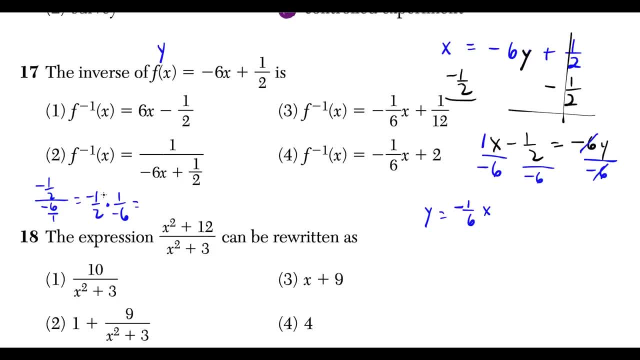 And we have a negative times. a negative is positive and then 1 over 2 times, 1 over 6 is 1 over 12. So if you can't do that part in your head, Just do keep change, flip on the side and that's going to get us here and now we could just match this, our inverse. 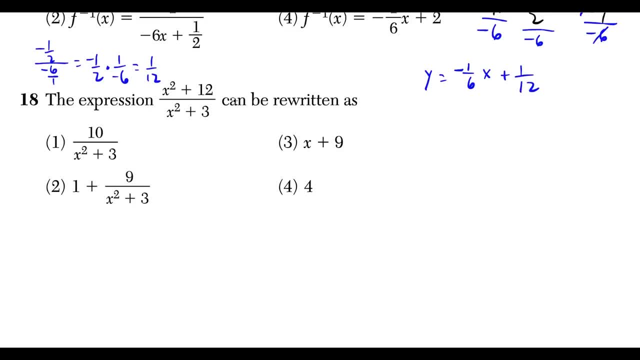 Function is going to match to choice 3, question 18. we could do polynomial division, But there's a cooler way to do this and to do this question: the slick way. Just know, when you have something like a plus B over C, That's the same thing as this. you could say a over C plus B over C. 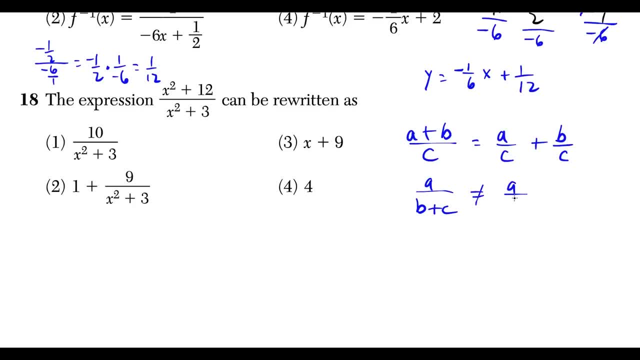 however, please don't ever say that this is true. this is not the same thing as this, and That's this. algebra is not allowed. This is perfectly fine, So this one. what jumps to mind right away is just rewriting the top as x squared plus 3. 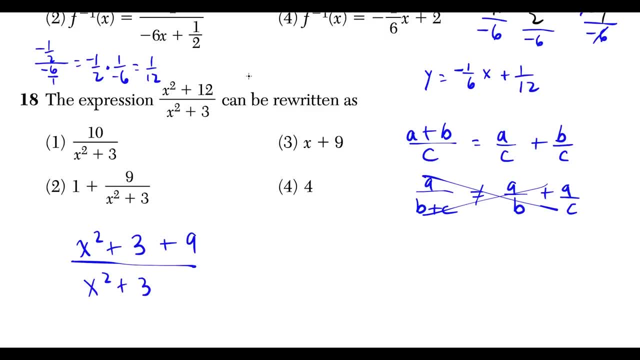 Plus 9, like this: over x squared plus 3, and then what I want to do is I'm going to break this into two fractions, so I'm going to call this first x squared plus 3 over x squared plus 3, and then I'm going to 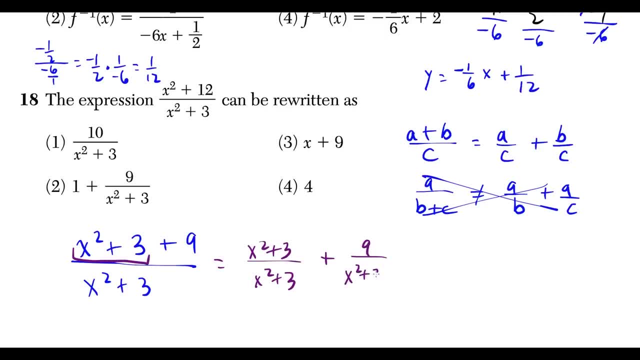 Separate the 9 into a separate fraction like this, where once again I'm just using this property of algebra and now this simplifies really nice: x squared plus 3 divided by itself is 1, So I get 1 plus 9 over x squared plus 3, so this is going to match to choice 2. 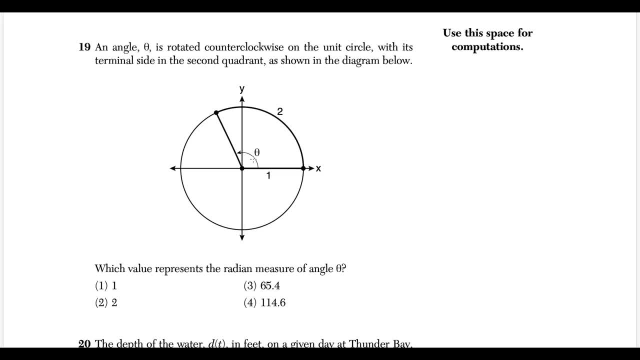 Question 19 is so easy that it's difficult. We're given this diagram for angle theta on the unit circle And we want to know which value represents the radian measure of angle theta. so for this one here, Just know, when we're talking about radians, this refers to the intercepted arc. 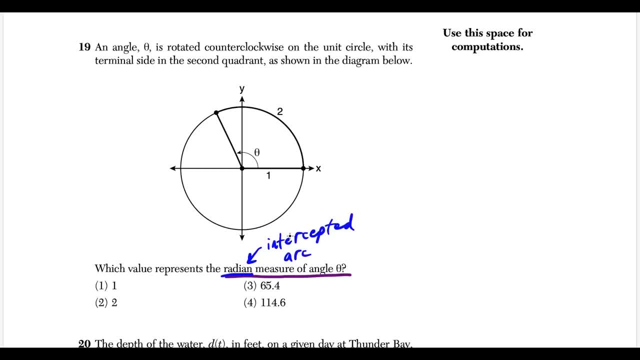 on The unit circle. so this is how radians are defined. it talks about the measure of the intercepted arc on the unit circle. So the reason I say this question is so easy that it's difficult Is that the measure Of the arc that's intercepted by theta is equal to 2, and that's simply our answer. now to convince you of this. 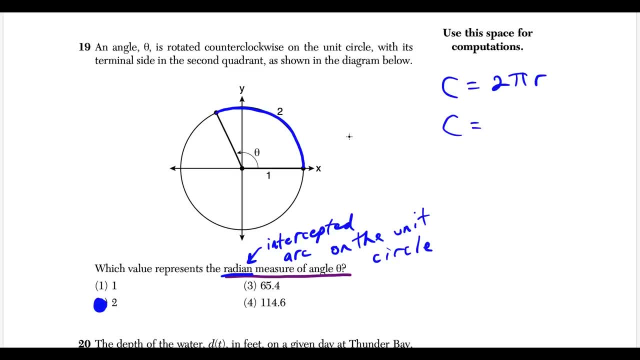 Circumference in general is equal to 2 times pi times r. so if I'm on the unit circle, I have a radius of 1, my full circumference would be 2 times pi times 1, which is 2 times pi and 2 pi a. 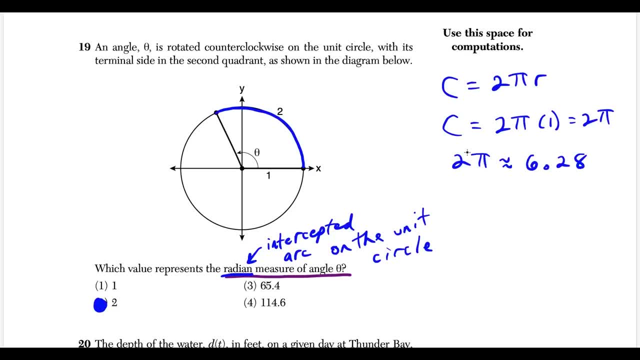 Bad approximation would be to say 6.28. if I did 3.14 times 2 and notice that if the whole spin is 6.28 ish, This spin- roughly 1 third of it- is equal to 2. so that's how. I'm 100% sure here that the measure of angle theta in radians. 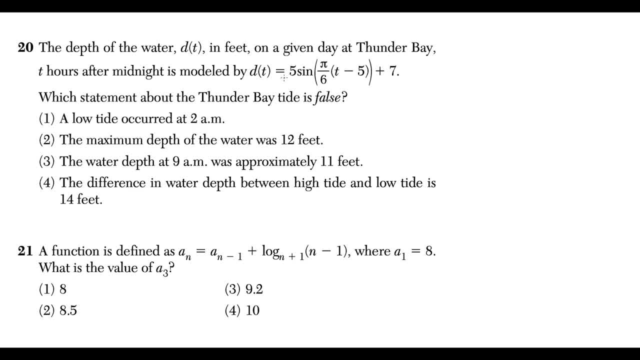 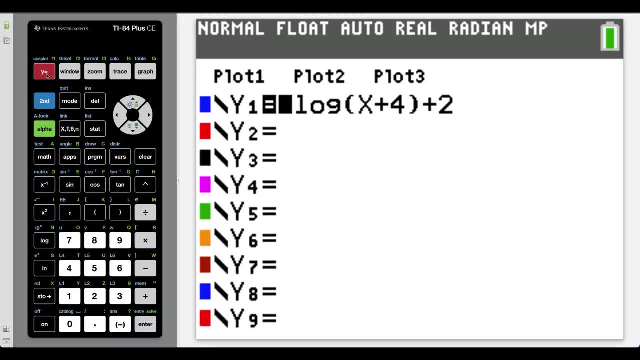 Is going to be equal to 2, question 20?? We're talking about the depth of water in Thunder Bay And we have this function here for the depth, and before I look at any answer choices, Let's just get a graph of this. so we'll go over to the y equals. 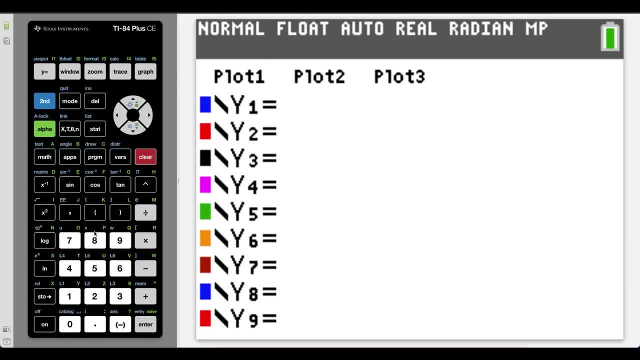 And it's very important that we stay in radians for this one- and what we have is we have 5 Times sine and then in front of our parentheses we have pi over 6, so we have pi over 6, And then we're going to open a new set of parentheses and t minus 5. we could just write x minus 5. 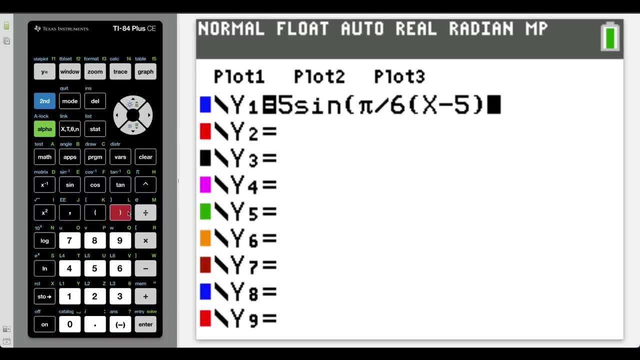 We have to close the parentheses around x minus 5, and then we have to close it Around the argument of the sine function. then we could tack on our plus 7. So just make sure your parentheses are good, because it could throw off the whole question now when we press graph here. 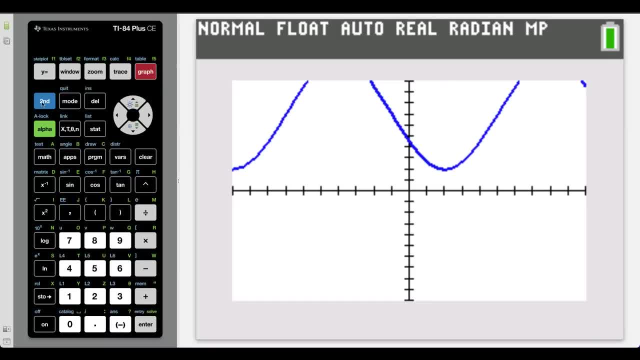 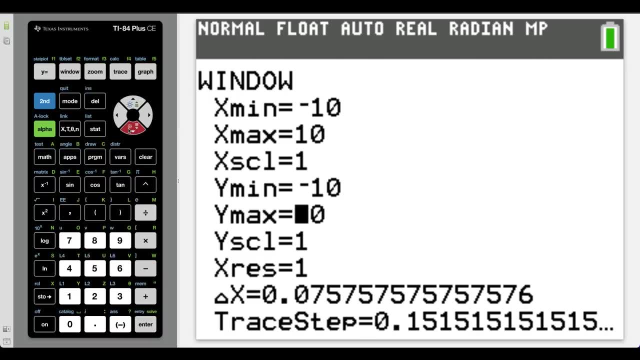 You don't really get the best picture of what's going on. so What I would do for a question like this is I would adjust the window and let's say I go up to a y maximum of 20. So we play this game here and notice that it gives us a good picture of what's going on. 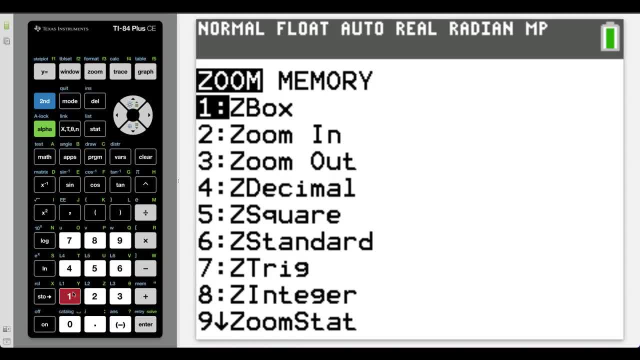 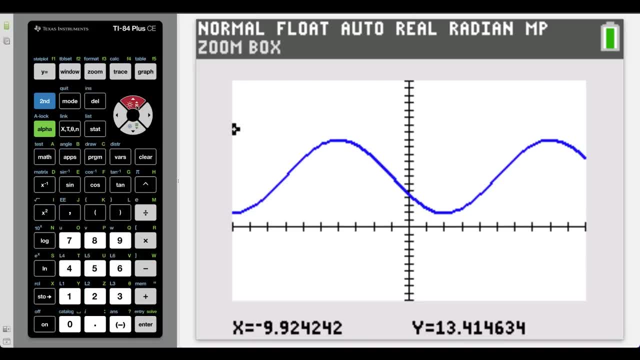 But another nice little trick for zooming: you could press zoom number one, Zoom box, and if I scroll out here like this It's kind of like cropping a photo when you use zoom box. you could press enter. So let me just make the space here. I press enter once. 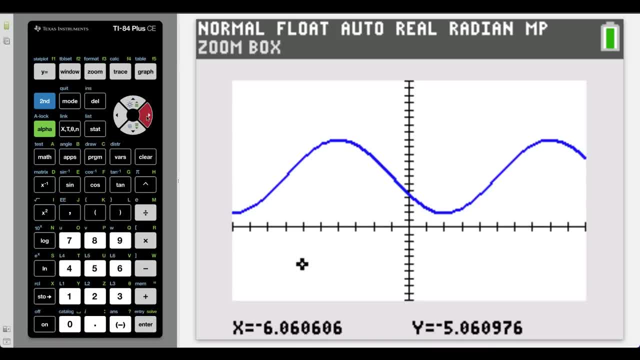 I'm going to drag this down and then I'm going to drag it across and notice here that it's making our rectangle. So let me try that again. zoom number one, because that actually didn't look like anything was happening, So I'm going to press enter once. 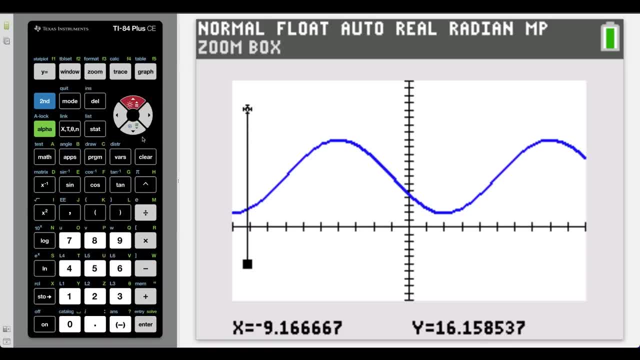 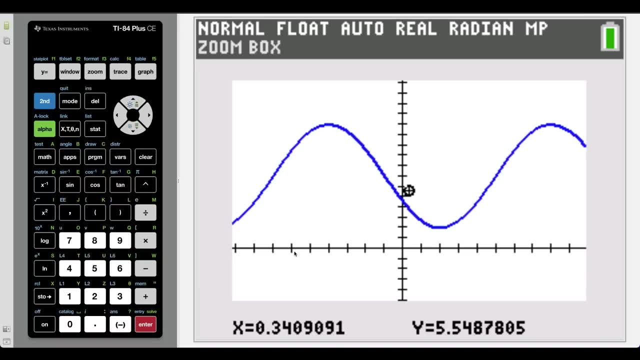 And then I'm going to go up here It is. so. this is much better and I drag it across and once again, It's just like cropping a photo, so that's going to give us this picture here And this is what we'll borrow to go through our answer choices. one other thing. 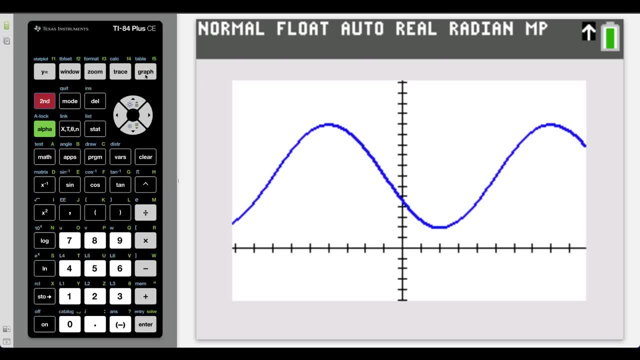 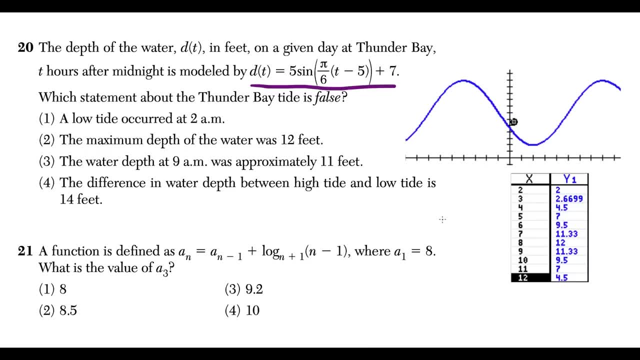 We could borrow to was: let's get a table of values. So if we look at the graph here, We press second graph and we could scroll around. what we could do is: we have the picture, But let's go ahead and borrow some of these values here. So this table will be useful just in case we don't feel like counting too much. so we have a low tide and remember we. 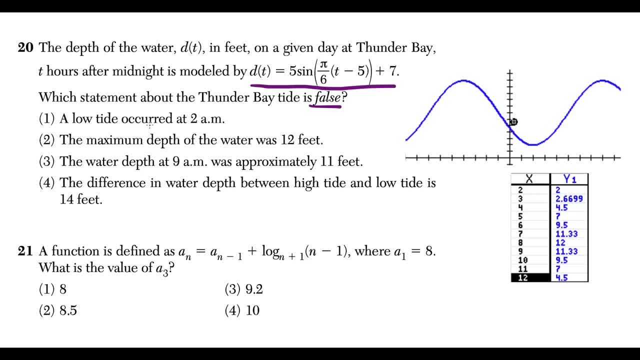 Want to know which statement is false, so don't just say, oh, this is true and pick the wrong answer. That would be very depressing. so we have a low tide occurred at 2 am, So at t equals 2. notice. This is a low point here, so this one's a true statement. 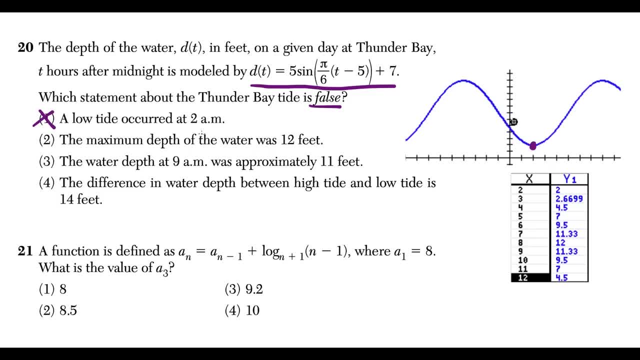 So that means we're going to exit out because we want the false one. the maximum depth was 12 feet and if we look here, It looks like the biggest number in the list is 12, and let's just make that a little bit finer here. 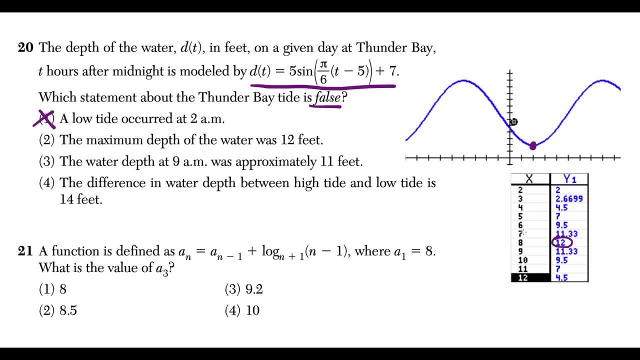 So I'll make this smaller. So this is our biggest y value: 12- and it occurs at t, equals 8. so if we count out here, notice We're going at 1, 2, 3, 4, 5, 6, 7, 8. so this is also a true statement. the maximum depth: 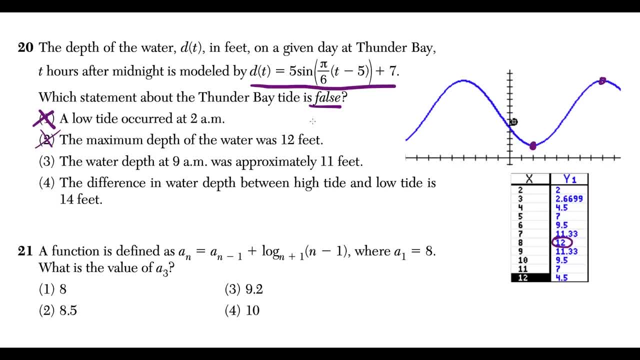 Was 12 feet, and that occurs at t equals 8 hours after midnight and now we have the maximum depth. I'm sorry, the water depth at 9 am Was approximately 11 feet, so look here at t equals 9. so t equals 9 gives us: 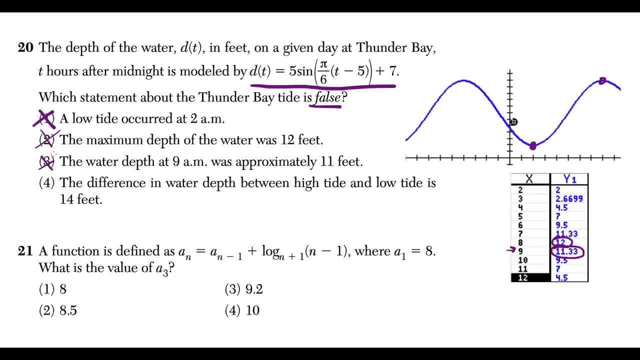 11.33, which- this is a nice statement here- approximately 11 feet. 11.33 is pretty close. Now the last one here is looking like the false one, just by a limit. So I don't want to be dominating all the others, But let's see here: the difference in water depth between high and low tide is 14 feet. well, if we look here, low tide was at 2. 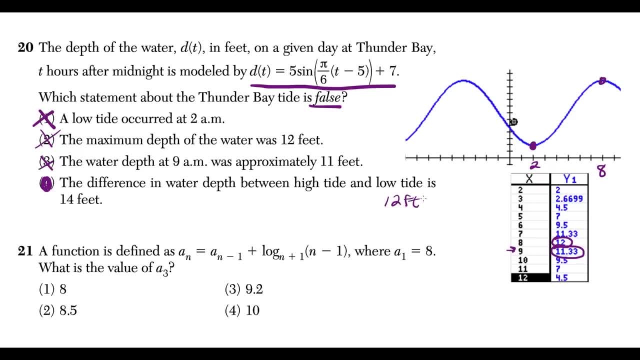 High tide was at 8 and if we do 12 feet Minus at t equals 2. we had a depth of 2 feet. the difference should be equal to 10 feet, But they're saying here It's 14 feet, so that's why this statement is false. so definitely choice for so question 21: 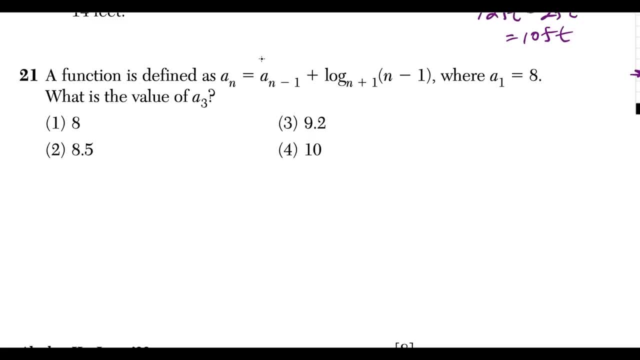 We have a nice recursive function and I know it's recursive. We have a sub n and a sub n minus 1 represents the term before a sub n. so here We're starting with. a sub 1 equals 8. so when I want to find a sub 2, this refers to when n is equal to 2. 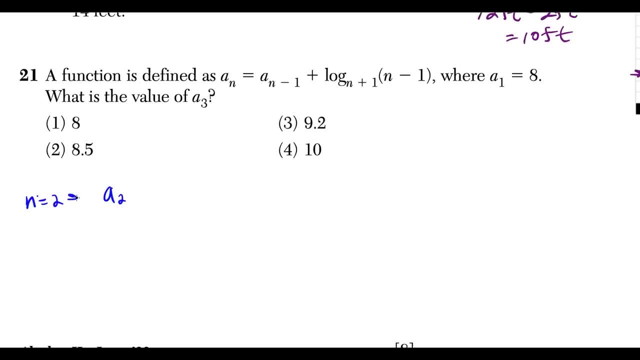 So let me just make this much neater. so we have n equals 2 and that would give us a sub. 2 equals a sub, and if I plug in 2, I get 2 minus 1, which is 1, and I have plus log base and 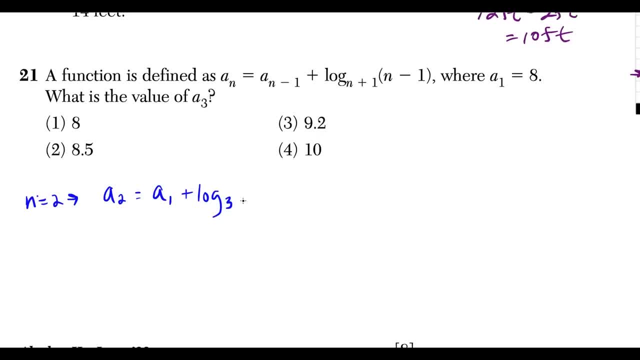 Once again, if n is equal to 2, 2 plus 1 is 3. so I have log base 3 of and if we plug in 2, we get 2 minus 1, which is equal to 1, and This is going to be equal to a sub. 1 is 8. 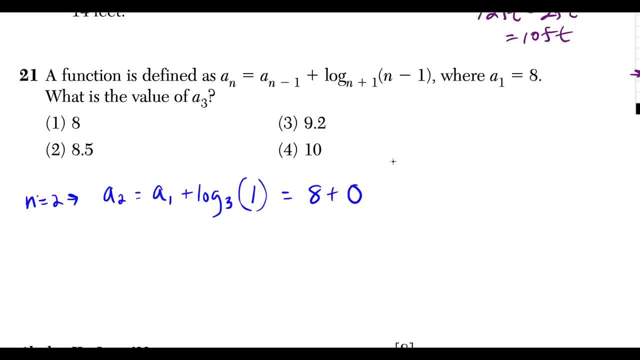 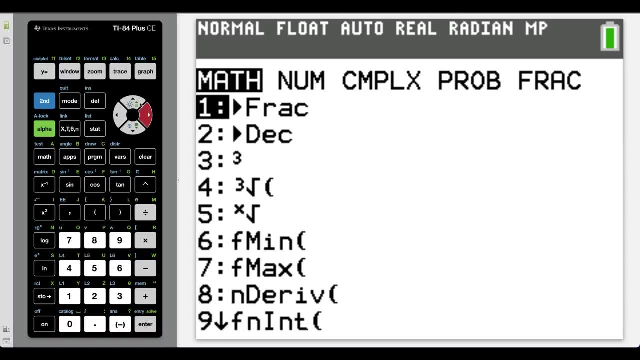 Plus, and log base 3 of 1 is equal to 0. you could use the calculator to check this out. So if you don't know how to do logs in the calculator, you press math, you go up And I got to get out of fraction. so math up. log base is letter a here and 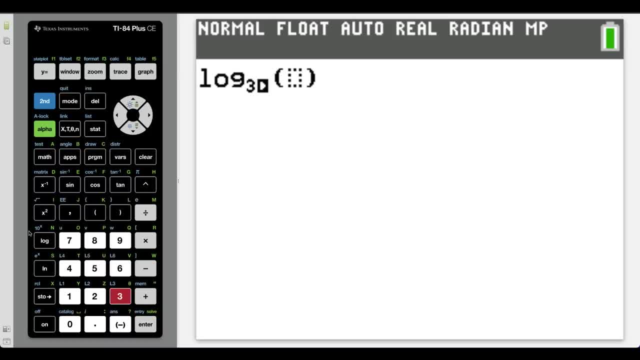 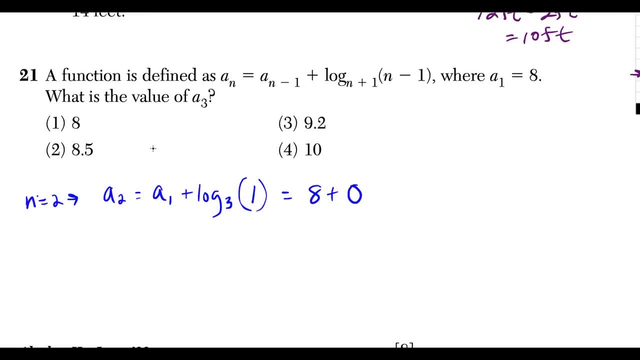 The reason why we go to this one is when we have a base like 3, There's no button on the side for that, so we have to make a custom one and log base. 3 Of 1- we can see here- is equal to 0, so I'm able to do this in my head though. 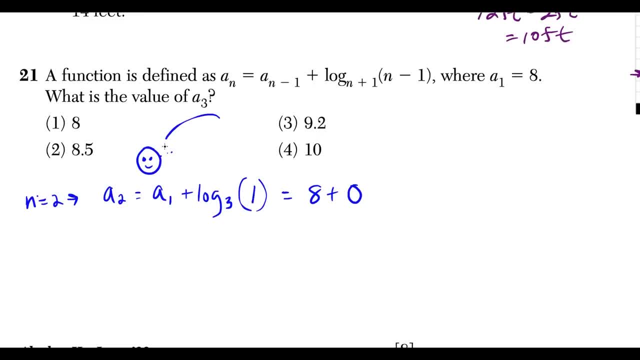 And if you want to see a little trick for doing these in your head is I turn the log into exponent form. so the base is 3. so I say in my head, 3 to the blank power is Equal to 1. and I know that 3 to the 0 power equals 1. so that's how I know. 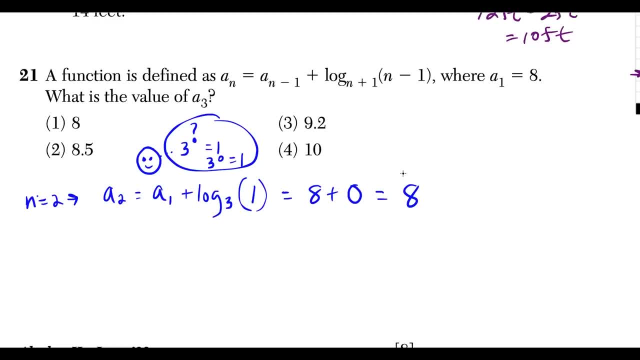 This simplifies to 0, and then 8 plus 0 is equal to 8, so that's a sub 2. So now, when I want to find a sub 3, that's when n equals 3, I'm going to get a sub 3. 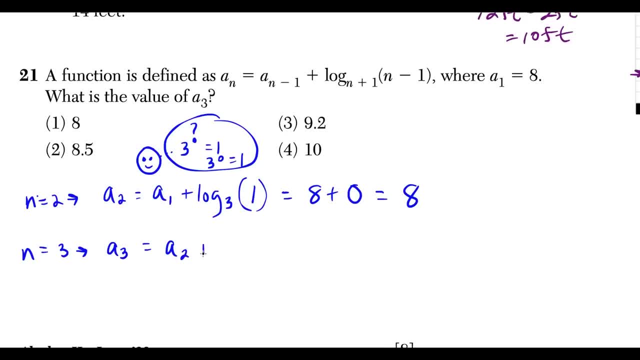 equals. and now I have a sub: 3 minus 1 is 2 plus. and then we have log base. we have n plus 1, so 3 plus 1 is 4, and now what we have is we have 3 minus 1 going here and 3 minus 1 is 2, and 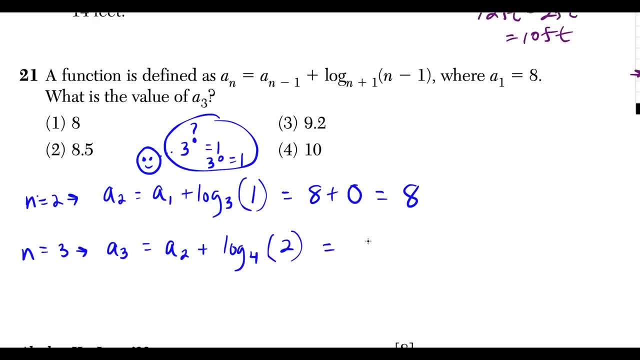 This is going to work out to a sub 2. we already said was 8, so we have 8 plus log base 4 of 2, So we could evaluate this part in our head: log base 4 of 2. what I'm thinking of here is- I'm saying 4- 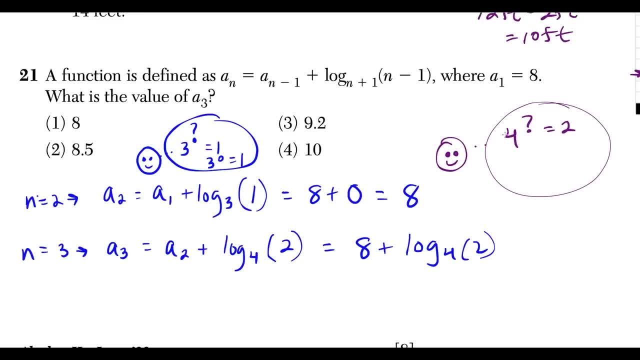 To the blank power is equal to 2, so I know we have to make the base smaller. so that means our exponent is going to be a fraction here and This we could say it's 4 to the 1 half power, because 4 to the 1 half is the same thing as the square root of 4. 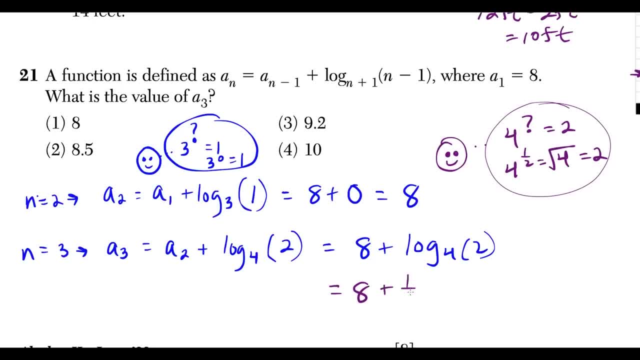 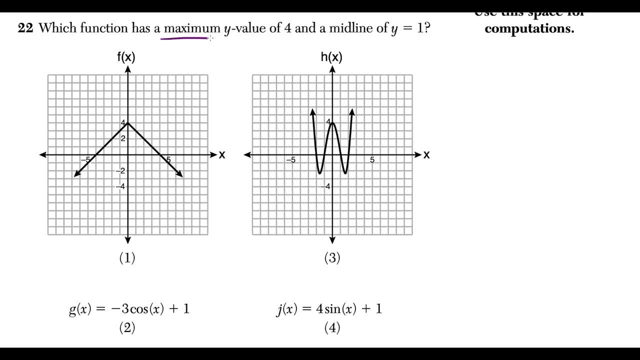 Which is equal to 2. so this is going to work out to 8 plus 1 half, and 8 plus 1 half, I could say, is 8.5, which matches choice 2. question 22: we want to know which function has a maximum y value of 4 and a midline of y. 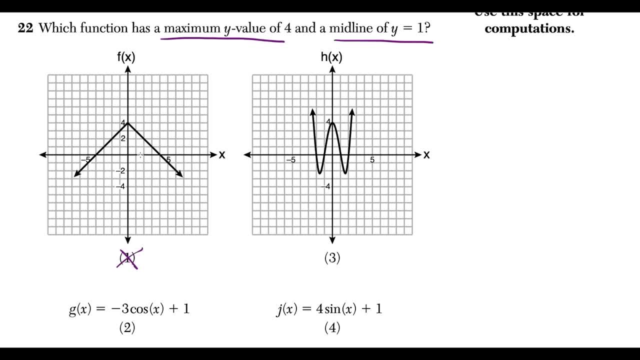 Equals 1. so right away I could eliminate this graph that they gave us because, yes, We have a maximum of 4, but if we look here at y equals 1, This is not going to count as a midline, because while we're going three units up from the midline here, 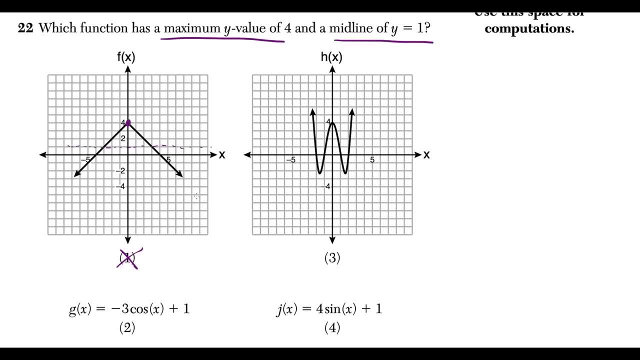 We're going to go infinitely south in this direction here, away from the midline. So there's no real nice equidistance from the midline and graph in the graph and choice one. So this one's out and for this one here, This one doesn't have a maximum y value of 4 because we have arrows going this way. 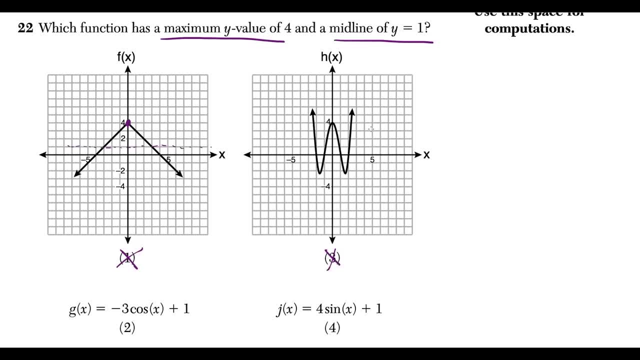 So this graph is just going up, up up to infinity. So this doesn't have a max value of 4. so that means we're going to do a little bit of legwork Here and graph the graph in choice 2 and choice 4. so for g of x we want negative 3. 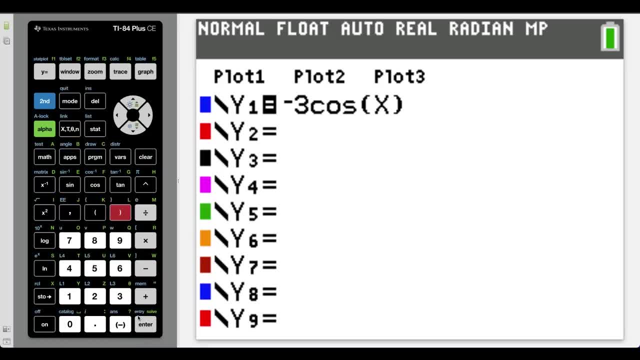 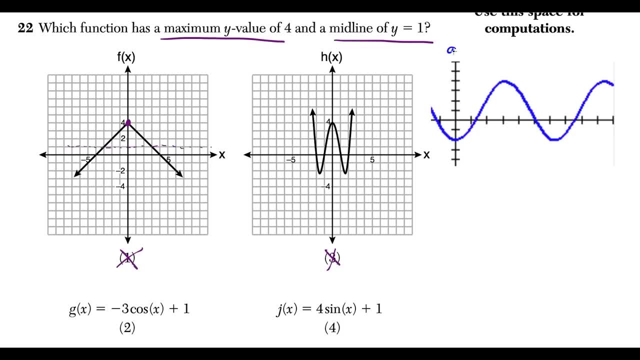 Cosine x, and let's make sure we get out of this, because it's cosine x with the plus 1 on the outside. So here's our graph and we're just going to take a screenshot of this. so now We'll go ahead and label this as g of x. and now let's graph the second one, so j of x. we could say was 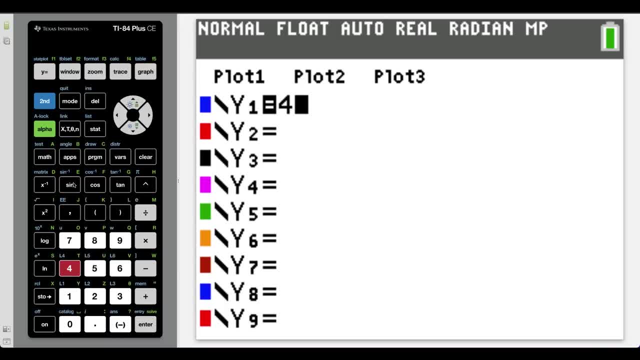 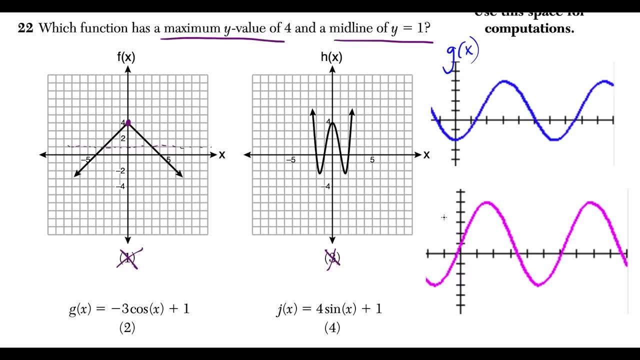 4 sine x. let's clear this out. We have 4 sine x, and Let's close the parenthesis around sine, And then we're going to tack on our plus 1, and we'll take a screenshot Of this graph as well. so one little change here. 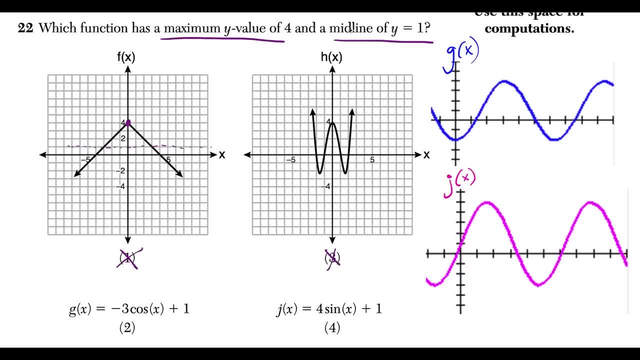 I'm just going to make this graph pink so that it definitely stands out. But now we're going to go ahead and run through the given conditions again. so let's start with g of x. We have a maximum y value of 4. so if we look at a point like this, 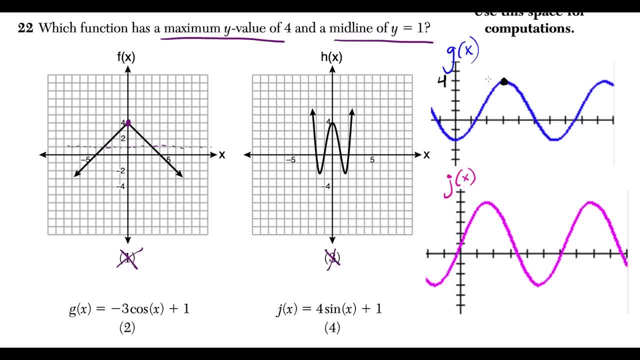 You can see how this lines up with 1, 2, 3, 4, so that first condition is met. And if we draw in a midline at y equals 1, you could see that This is acting as the midline for this trig function, because to get from the midline to this point up here, 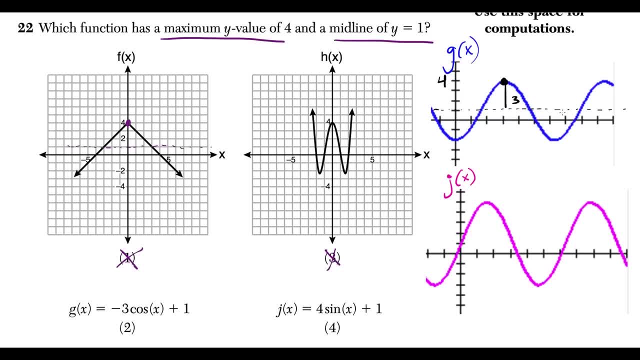 I'm going up 3 units like that, so there's a distance of 3 to this point. and then to get from here to here, I'm going from 1 down to negative 2, so that's a distance of 3 as well. So this is looking like our answer. now Why is choice for no good? well, right away. 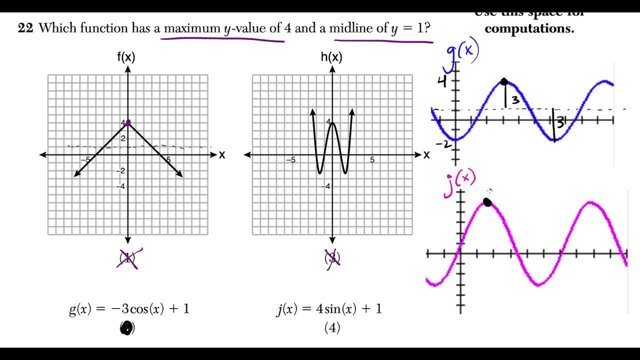 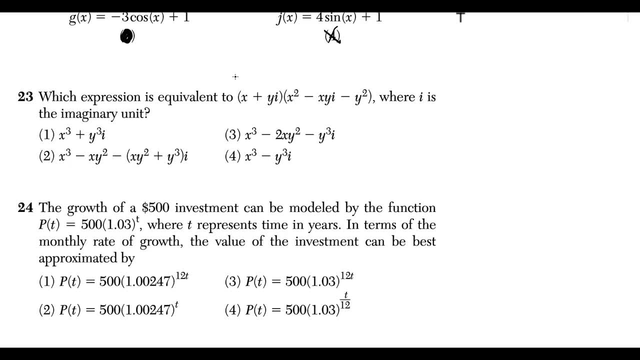 We could see we're going up 1, 2, 3, 4, 5. so this has a max value of 5, So it's automatically out. definitely choice 3.. I'm sorry, definitely choice 2. so for question 23, Just be good at distributing and know that I squared is equal to negative 1. 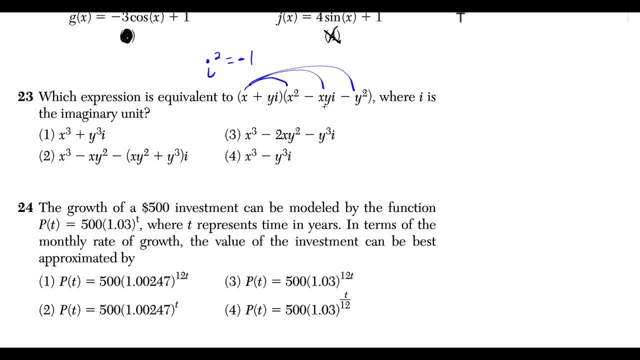 So I'm going to start by distributing the x. and if we distribute the x, x times x squared gives us x to the third, and then we have x times minus x- yi is minus x squared yi. and then we have minus x- Y squared. and then one thing I like to do when I distribute the next thing is I write like terms underneath each other. 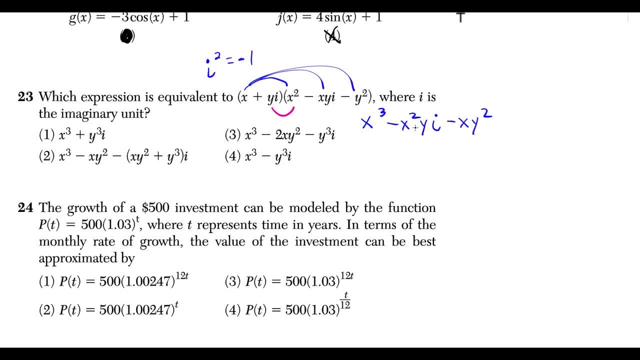 So here I have yi times x squared, and that's going to give us plus x squared yi. so right away, I see that these terms are going to cancel out. and now we have yi Times minus x yi, and that's going to give us- I'll write that over here- We're going to have minus x. 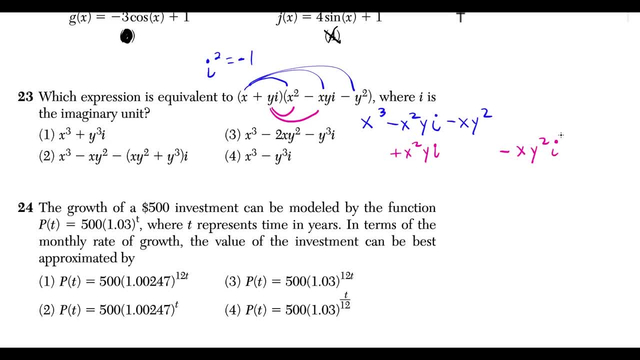 y squared and then I times I gives us I squared, and this is the part where we use that I squared equals negative 1, and then we have yi times minus y squared and That we could just say: yi times minus y squared is minus y. to the third: 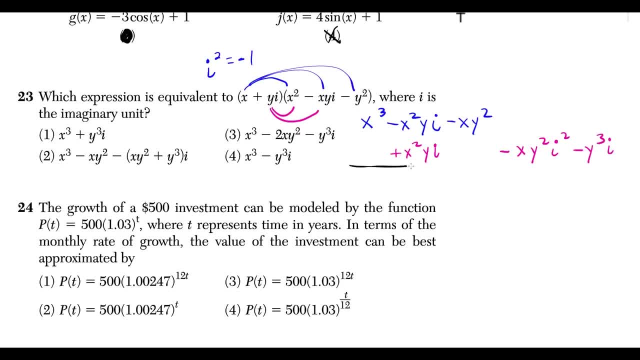 Times. I like this. so now we could just combine like terms, and once again these terms are opposite, So they're going to cancel out. so we have x to the third, Minus xy squared, and then this part: here, the I squared equals negative 1. So think of this as minus xy squared times negative 1, which would make plus xy squared. 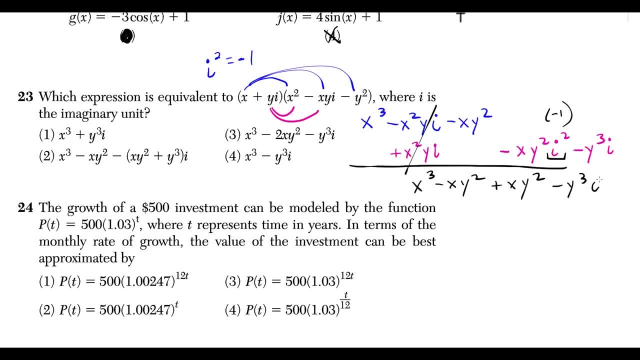 So that brings us here, and then we have minus y to the third times I, but notice that these are now opposite terms that could cancel. so this simplifies: to x to the third, Minus y to the third times I. so this is definitely choice for question 24, the final multiple choice question. 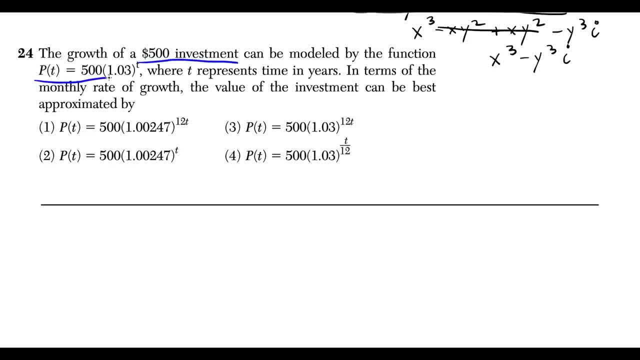 we have. the growth of a $500 investment can be modeled by this function, and t is the time in years- and This is the question- in terms of the monthly growth, In terms of the monthly rate of growth, the value of the investment can best be approximated by. so one thing. 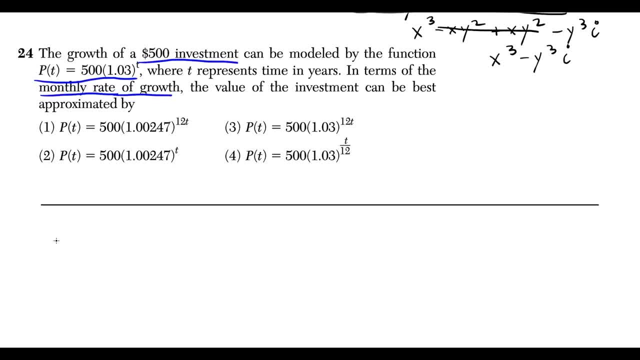 I'll tell you: this is not. do not. this is a very dangerous trap. do not think of this. So I'm going to say don't in all caps, because I'm not telling you to do this, But don't do something like this. like oh, 500 times 1 plus, and in this case, here the interest rate is. 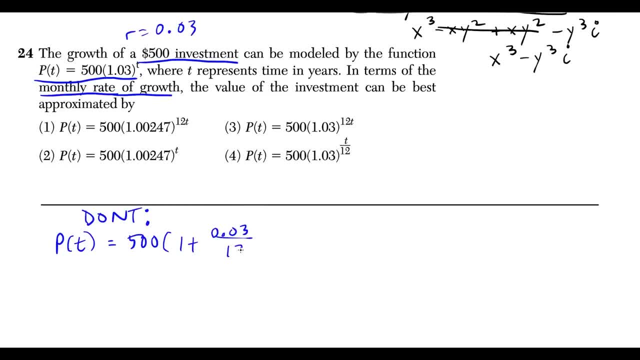 0.03, but don't say 0.03 divided by 12 to the 12t. this is a very dangerous Trap. it may not show up as an answer choice here, But it's a very, very, very dangerous trap because they're not telling us that this is compound interest compounded monthly. 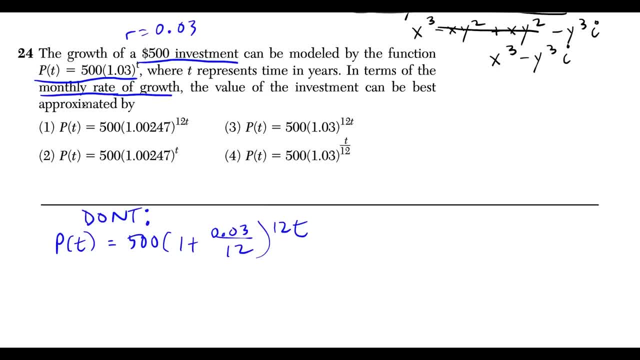 They're telling us to express this function in terms of monthly rate of growth. So this is not what we're doing here. We have to take a different approach here. so what we're going to do is We're starting with the function p of t, and p of t is 500. 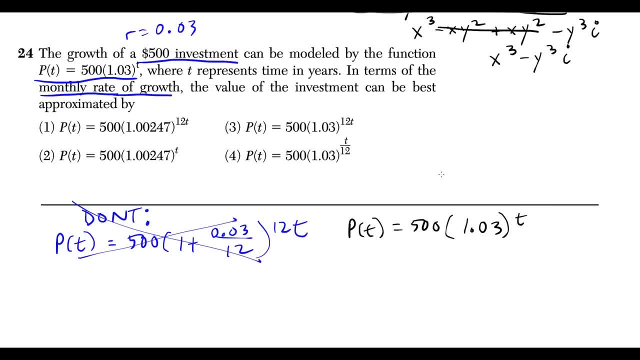 times 1.03 to the t power. so It's reminding me of this formula: p equals a, and then we have 1 plus the interest rate to the t power. so compound interest, Where we compound yearly, and in this case r is equal to 0.03?. 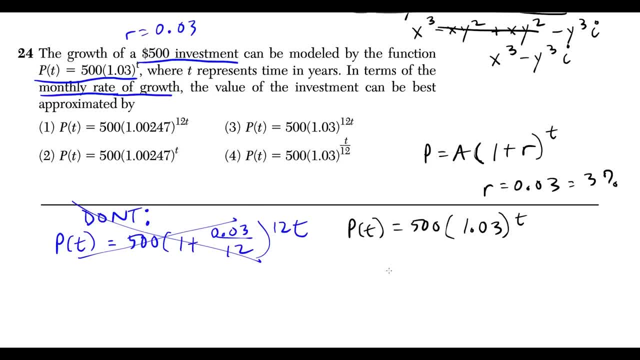 Which is the same thing as 3%. but what we're going to do is we're going to express this in terms of the monthly rate Of Growth. so we're going to use this property of algebra that, when we have a to the b To the c power, this is equal to a to the b times c. so what I want to do is I'm going to rewrite this. 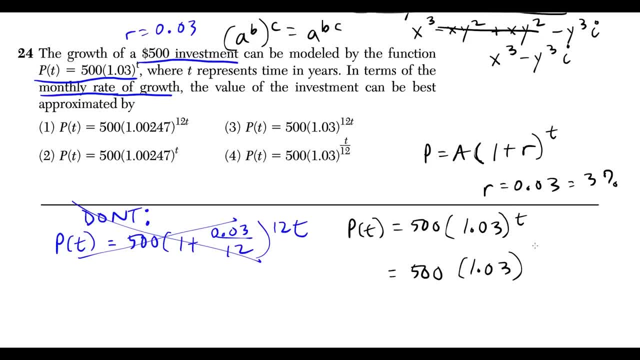 instead of to the t T power. I'm going to write this here as one over 12 times 12 to the T power. like this Now, the reason why I'm expressing it as a product, so that in a moment we could shift this over: 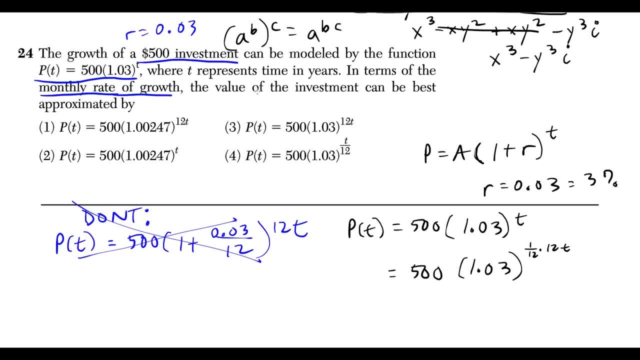 and express it in terms of the monthly rate of growth. So if we go forward with this here, what we're going to do is we're going to group this a little bit different Now. we're going to write this as 500 times 1.03 to the one over 12.. But I'm going to put this whole thing here in a 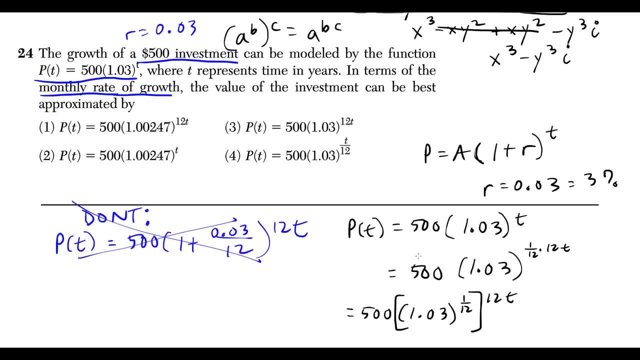 bracket and say this to the 12 T power. So you could see this is equal to the original. I'm not using this formula. I'm taking what we already have And I'm just shifting its representation. So now we could say: this is 500 times. whatever this works out, to which we'll write in a moment- 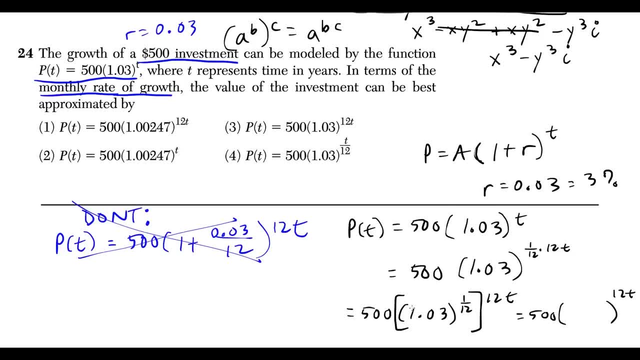 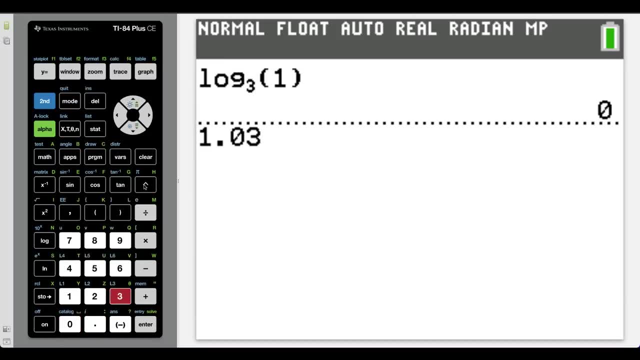 when we get the calculator going. But now we just have to evaluate what is 1.03 to the one over 12.. So let's go And do that. we have 1.03.. So 1.03 to the one 12th power, so one divided by 12.. And we could see here: 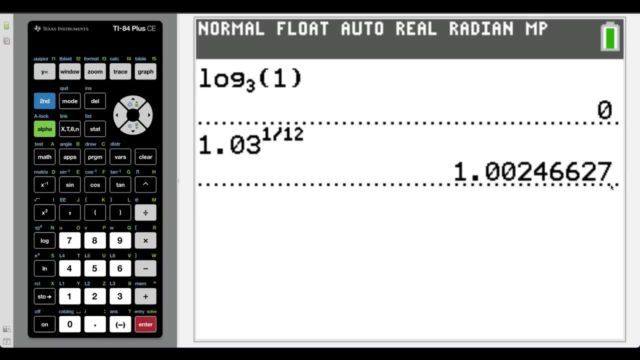 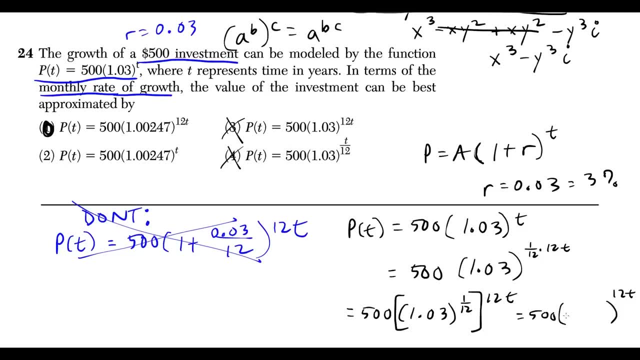 that we have 1.00246627.. And if we look, this eliminates choices three and four And this is going to match up with choice one because there's our matching decimal here. we said this works out to 1.0024.. And then if we round, it's going to round to a seven here. So this is definitely. choice one.